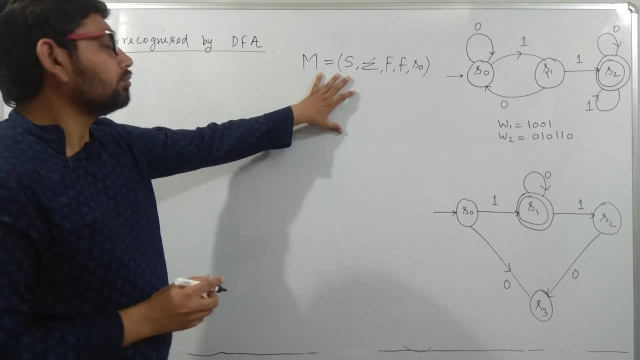 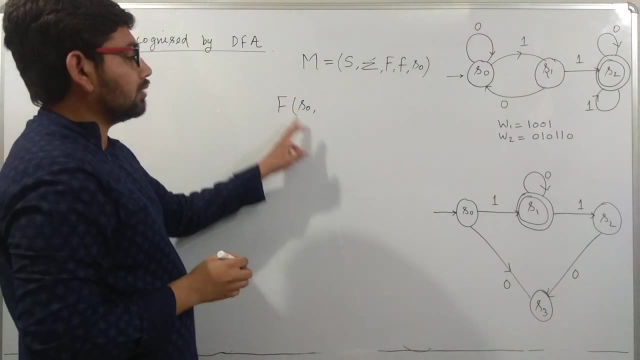 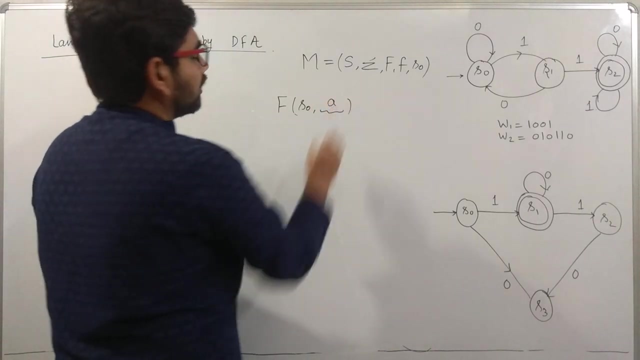 This is a deterministic finite state automaton. This is a deterministic finite state automaton. In this, when we were in S0 initial state to bring any transition in it, we gave it an input. So input can be a symbol of A form or a string of W. 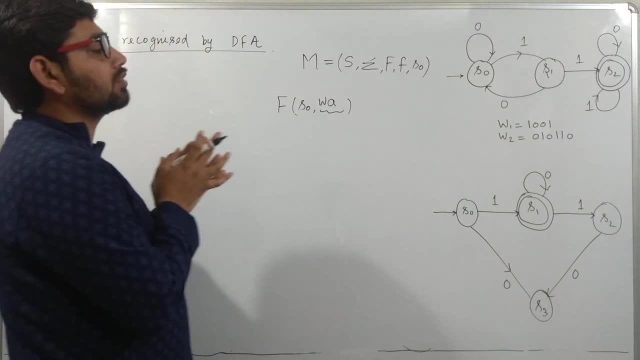 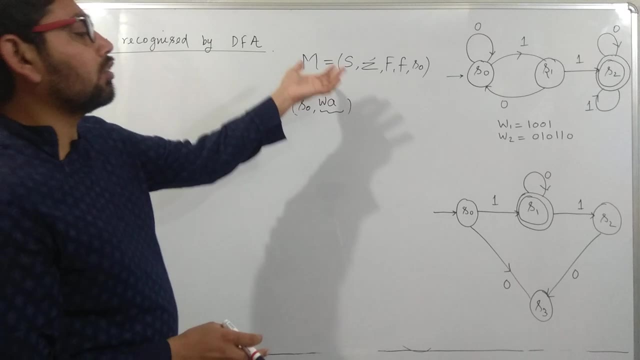 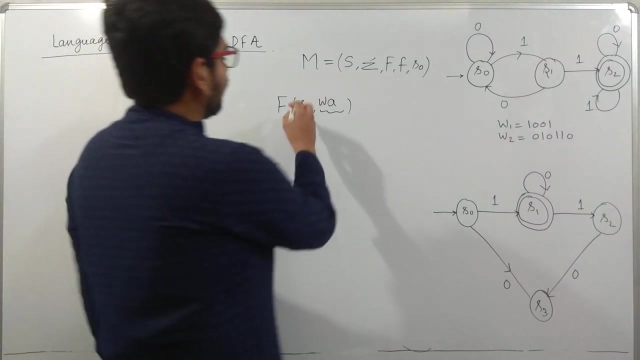 It can be any string made up of sequence of symbols, input symbols. So when we bring a transition in it, the machine, which is a finite state, automaton. finally we reach some state. So f is a transition function. So f to S is a function. 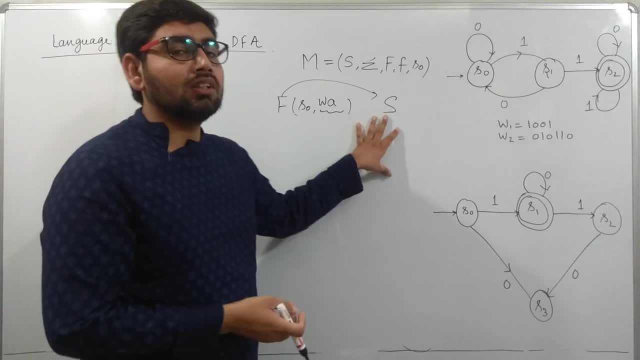 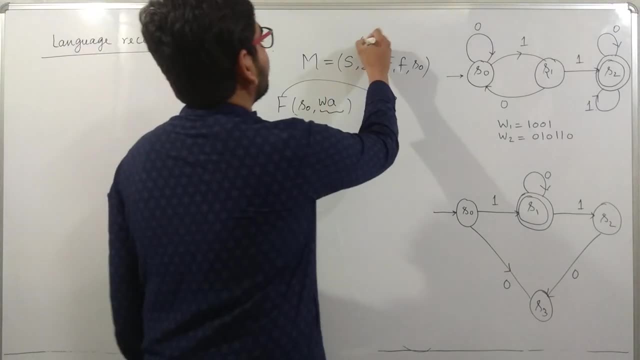 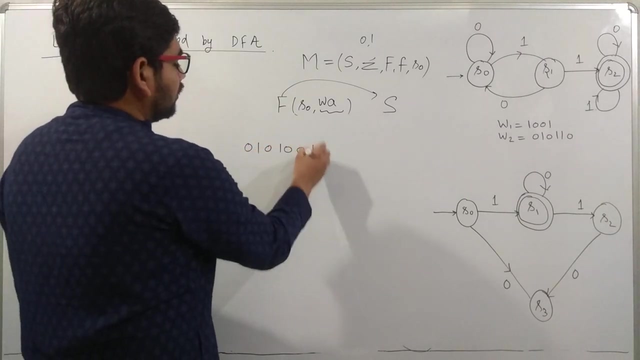 Finally we get a state, which is S state. Now we have some such strings If the input symbols are 0 and 1, 0 and 1 are two inputs, So string can be like this: 0, 1, 0, 1, 0, 0, 1.. 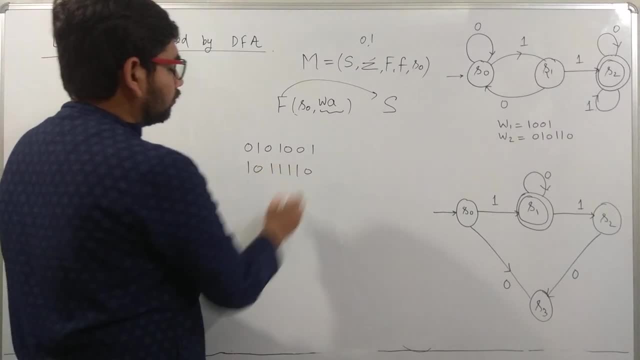 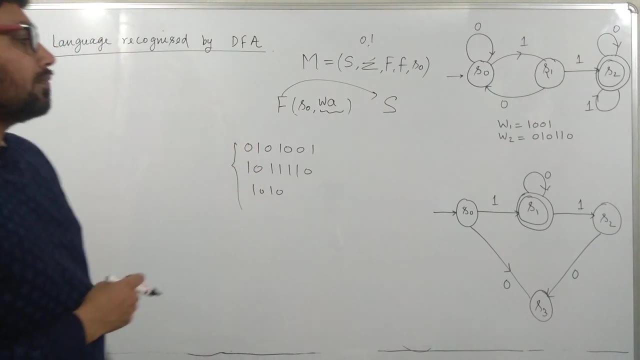 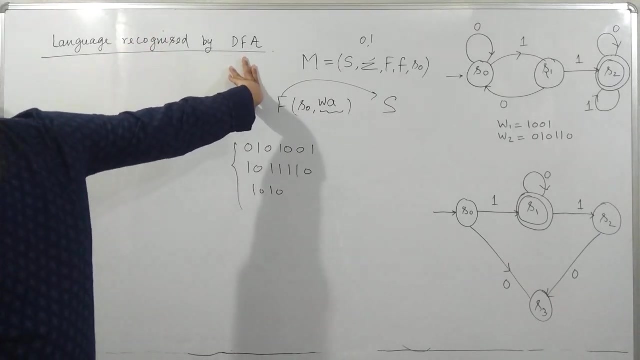 Some other way: 0 1, 1, 1, 1, 0.. 1 0, 1, 0.. Only this can also be So. the input strings can be different types of input strings. Now we want to see that our deterministic finite state automaton. 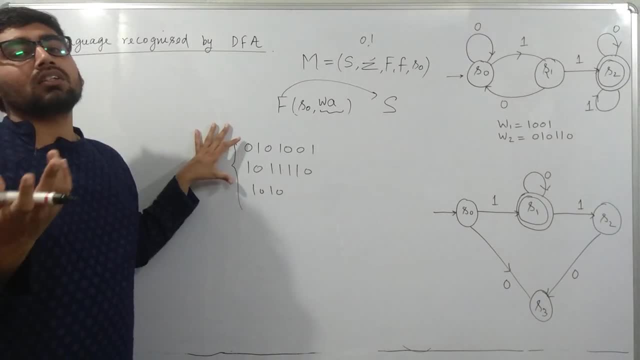 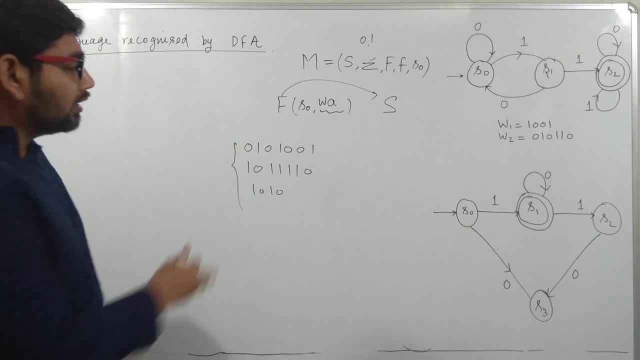 which type of input, which type of string it accepts And which type of string it does not accept, To which it will accept. What does it mean to accept? First we gave input to this finite state automaton which we had. First we gave input to 0.. 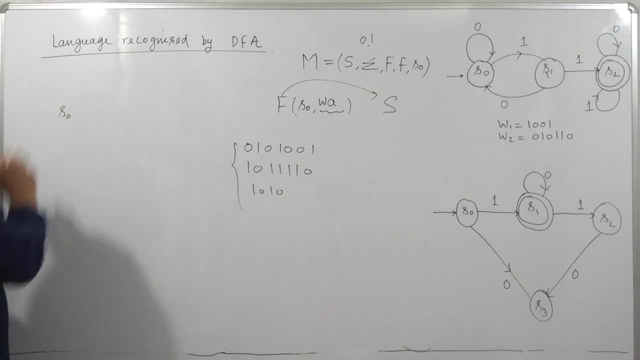 Suppose you were initially in state S0.. You gave input to 0.. You came to state S1.. Then you gave input to 1.. From 1 input you came to S2.. Then you gave input to 0.. 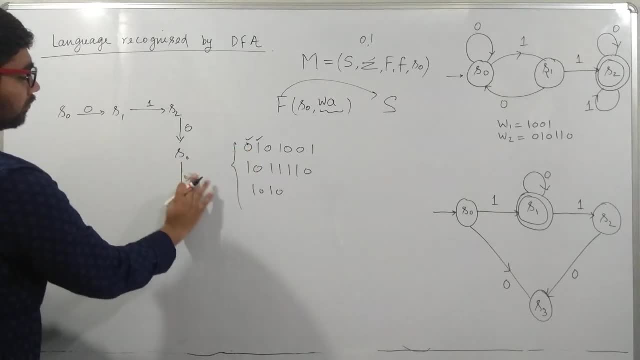 Then you came to S0.. Then you gave input to 1.. Then you came to S1.. So we will keep moving like this And when our string will be complete, we will give all inputs in string. So this will be our final state. 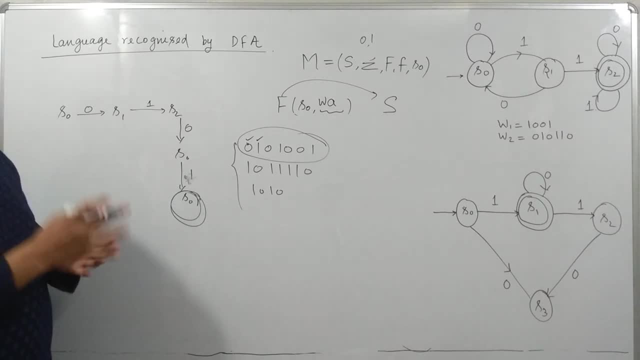 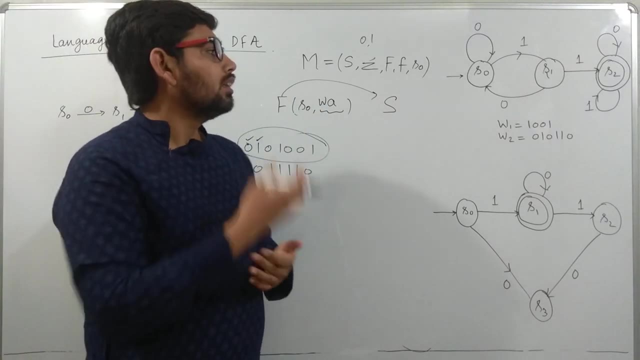 If this state is accepting state, Accepting state is already defined. We define that in finite state automaton, According to which we have to accept this string In which state we want to get this result. So we call that state accepting state. 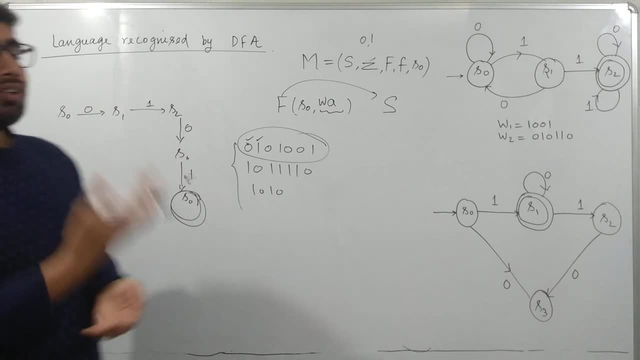 So accepting states are generally defined. We know that in which state we will get the result, So we will accept that string. So if it is finally ending in S0. And we are marking that S0 is accepting state Or 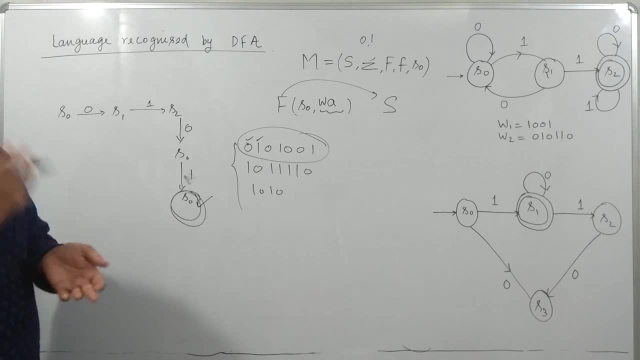 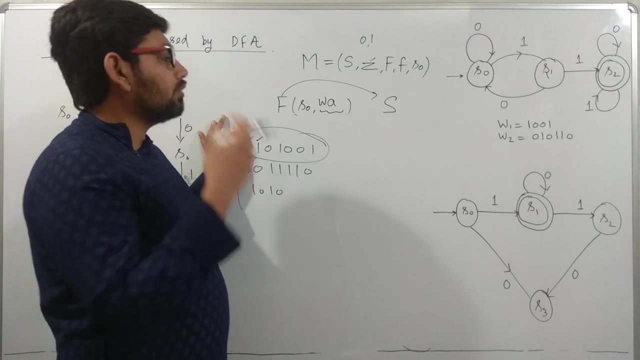 If it is recognizing state, So it is recognizing or accepting. So this input of our string, This input of our string, We will say that this is recognized by finite state automaton. This finite state automaton is accepting or recognizing it. 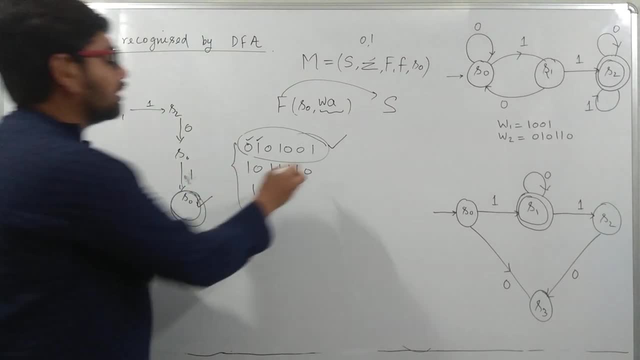 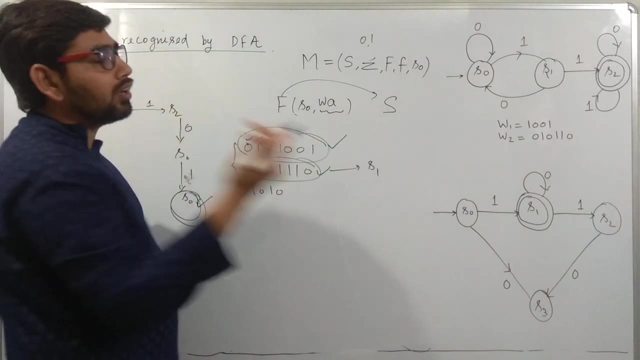 It is not rejecting it. And if we get such an input, such a string Which is finally ending in S1. And S1 is final state. Final state should be in F. It should be in F. F is such a subset. 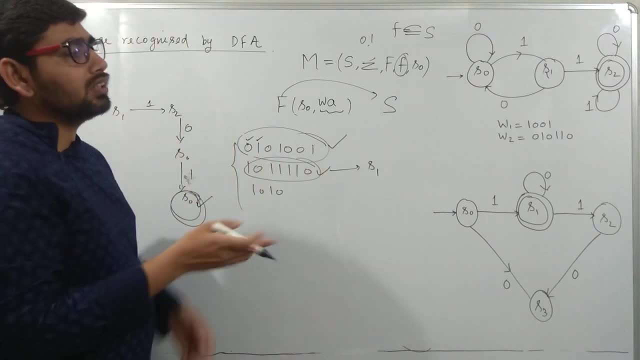 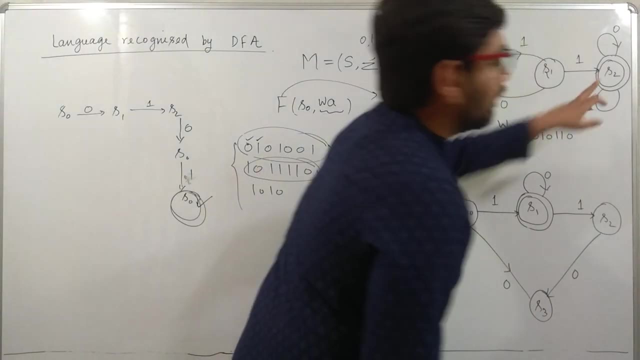 It has such states Which are final states, Which have double circles, As you have written these two examples. Now we will read about them, These two. This is the final state in this, This is in this There can be more than one final state. 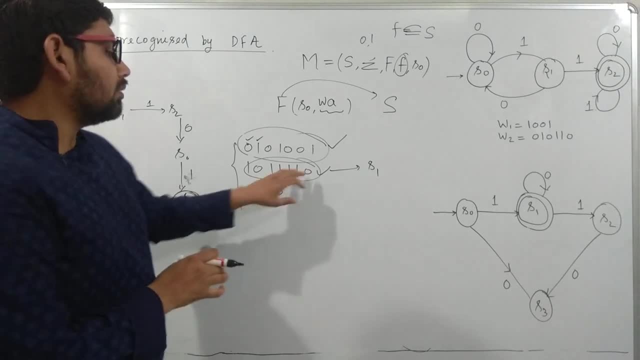 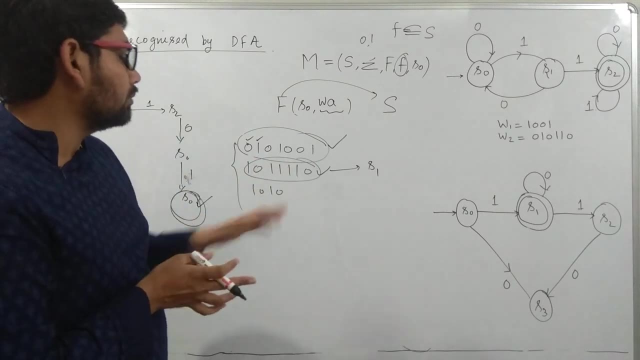 In a deterministic finite state automaton. So if we finally input this input, When we input this string In deterministic finite state automaton, So the final state we will get, If that state is accepting state, Then that string is accepting. 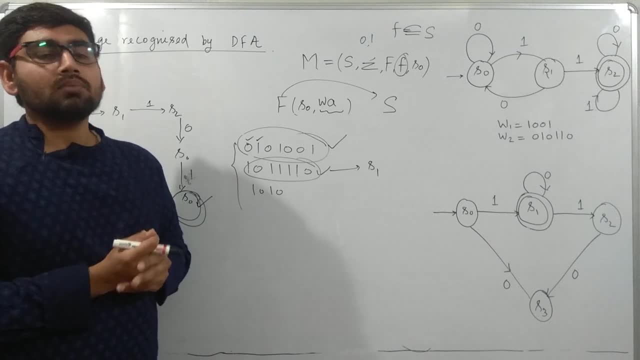 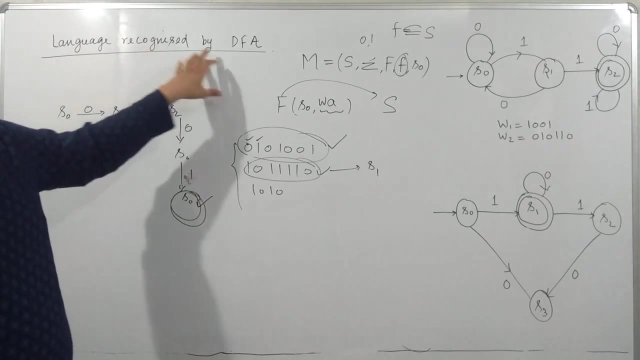 And if that state is not accepting, Then that string is not accepting. So that type of string is accepting Now which language is being recognized, Which language is being accepted, Recognized, or which language is being accepted From DFU. So the string which is being made from the input. 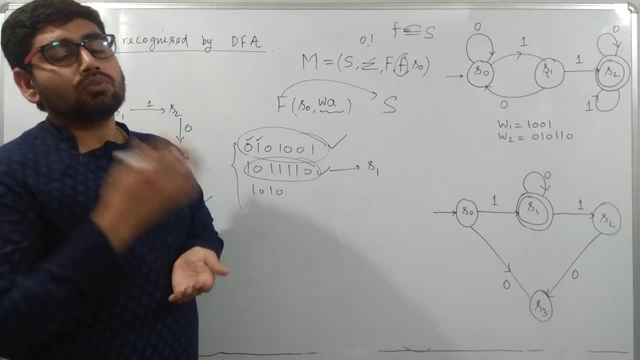 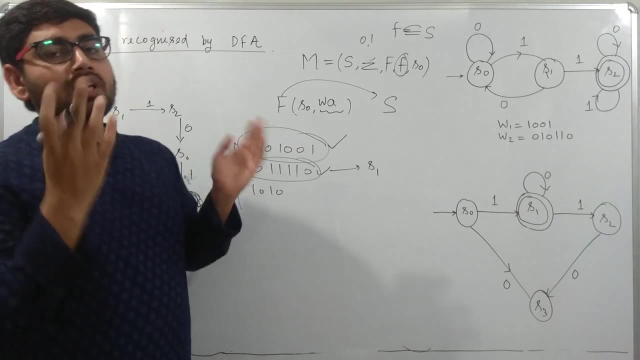 We can tell the type of string. We can decide that machine From that finite state automaton That this type of string will be accepted. This type will not be. So we define the language If we have m, Which is our deterministic finite state automaton. 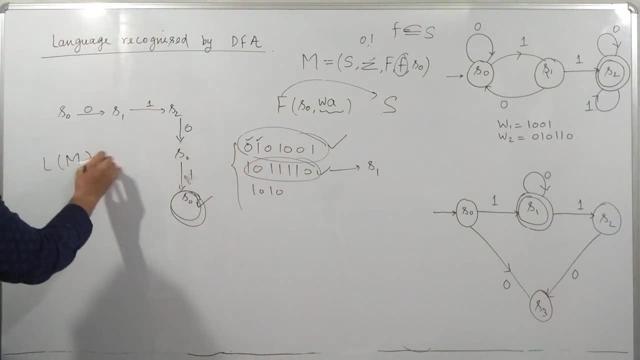 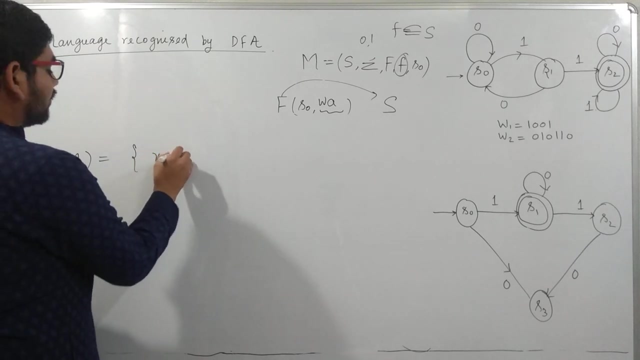 So we denote lm. We have lm Language recognized by Deterministic finite state automaton m. lm is language recognized Or language accepted by Deterministic finite state automaton m. In this There will be x type arguments Where: 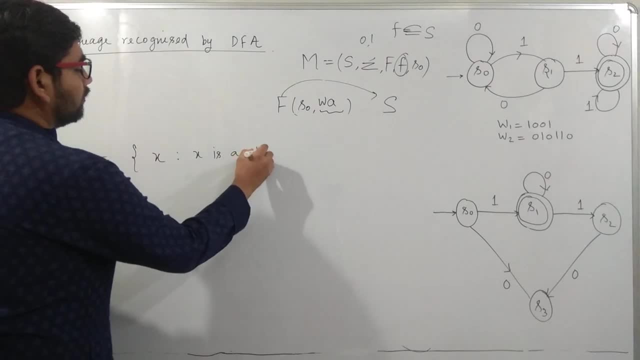 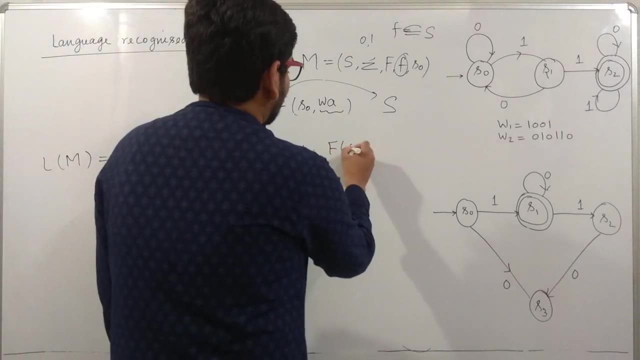 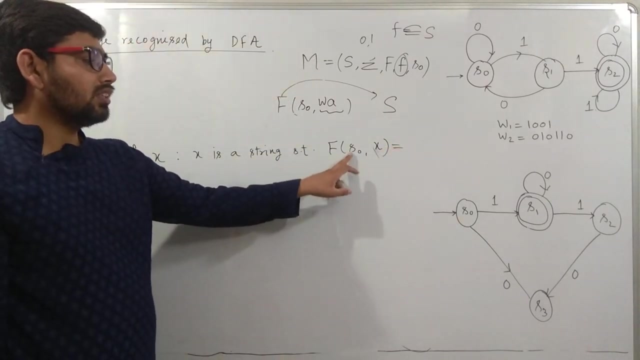 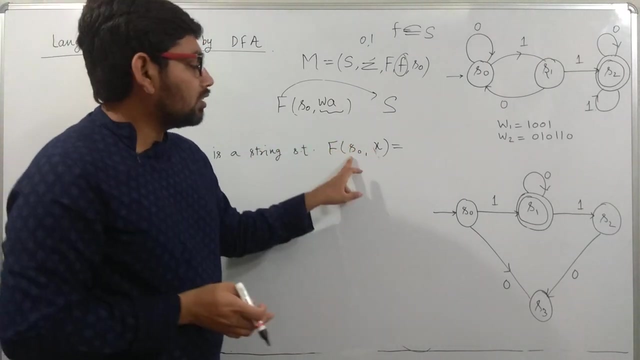 Where x is a string, Such that x is a string To which we, When Initial starting state, Will bring the transition By that string. input: Input the entire string, Because x is the entire string, Now the starting state. 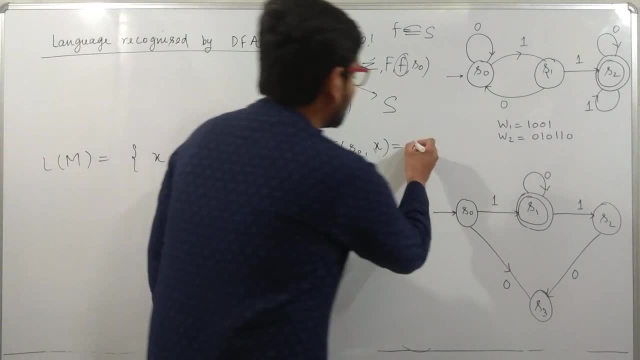 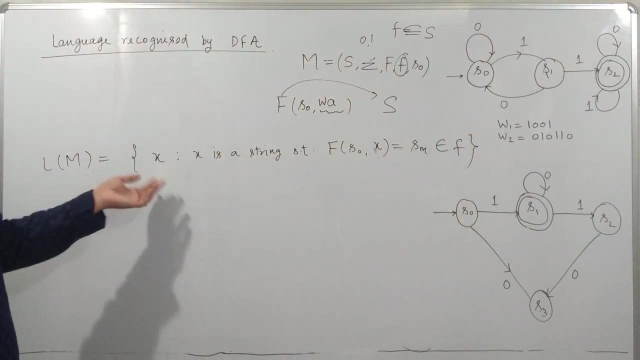 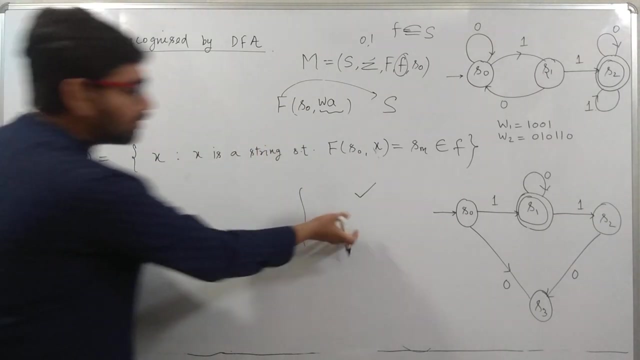 Let the string get the transition function, That from here. if it is accepting state, then we will say that x type string is accepting, so all strings of this type which are accepting. like we took three strings: first one was accepting, so it will block. second, one will not block. third, one will do. 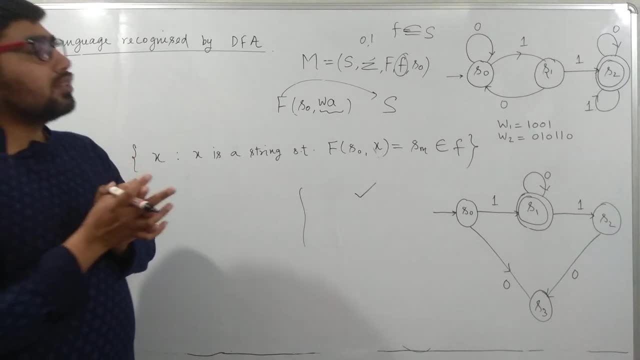 so all the string of input sequences which we will make, the input sequences which we will make from input symbols, or we can say string of inputs, those inputs which are accepting. accepting means that all the symbols in the input will be used in the input and transitions will be brought in the state. 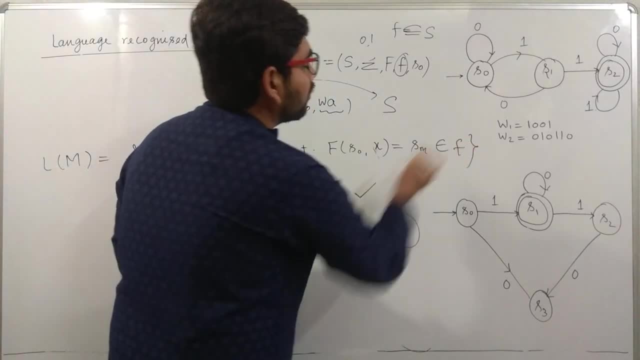 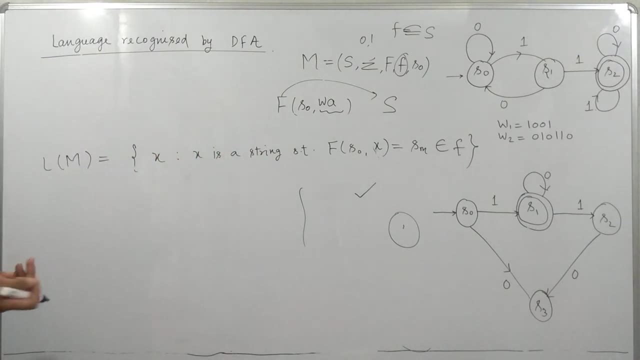 so the final state which we are getting is belonging to f or or or or or accepting state. so we will say that string is accepting and it will belong to the language that is a language of deterministic finite state, automaton m. that is a language that type. string is accepting means that is a language. 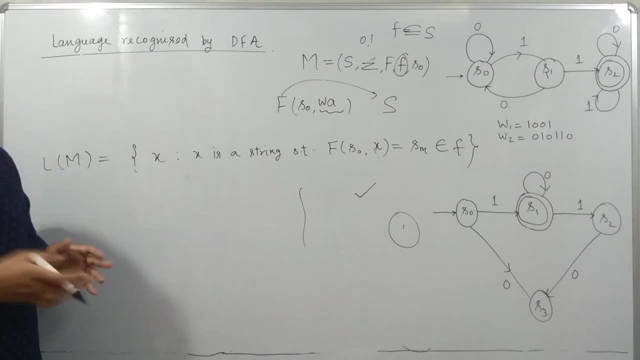 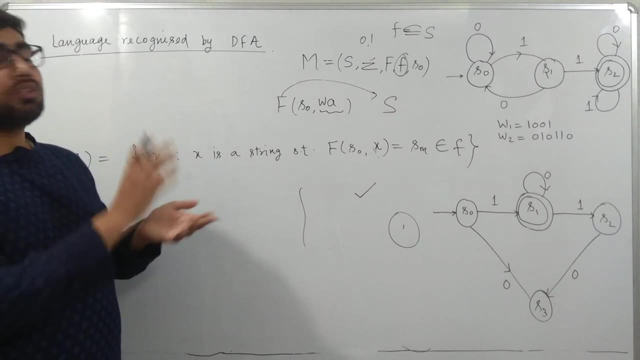 if someone does it again, then it is his language. so we will read some examples in this. we can decide that this type of string will be accepting and if not then it will not be accepting. so we can define it in set form and tell that this type of string is accepting. 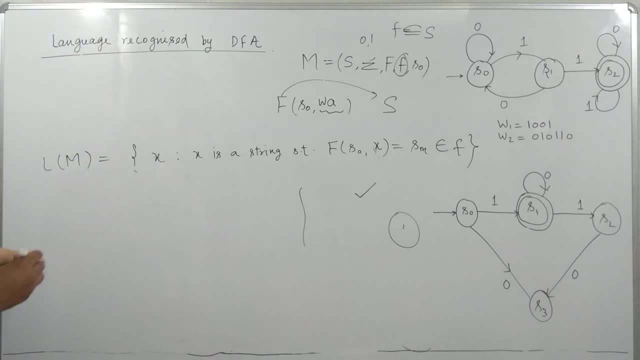 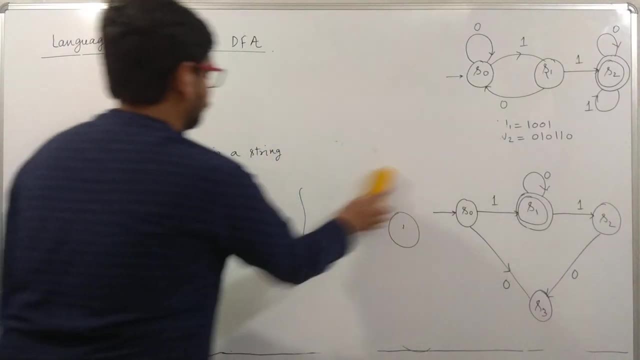 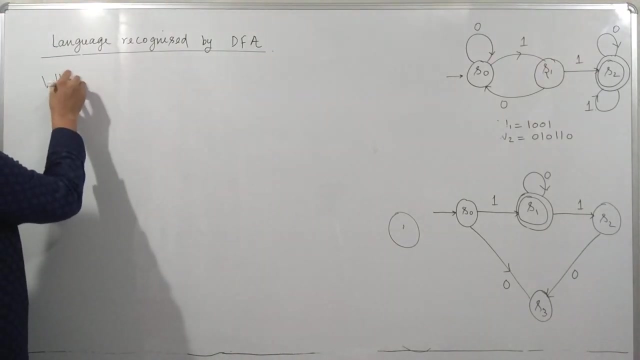 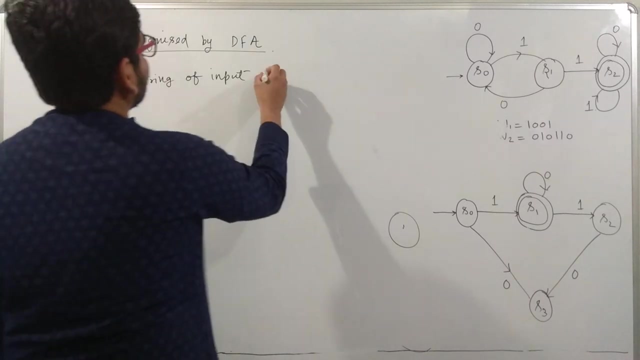 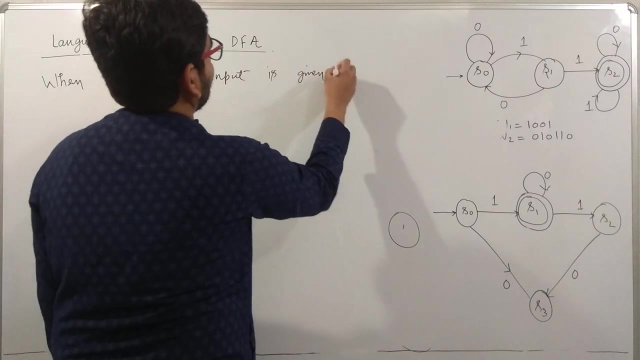 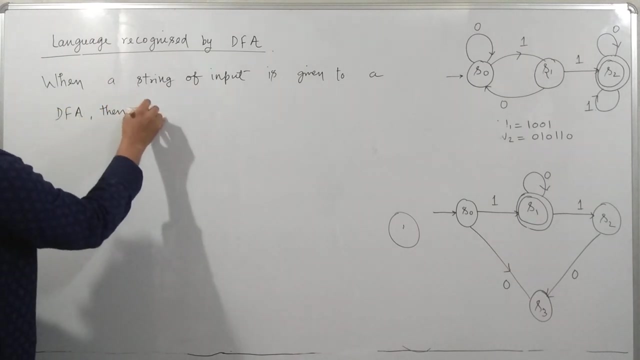 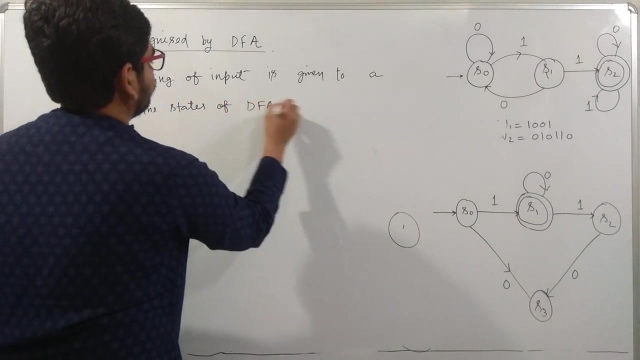 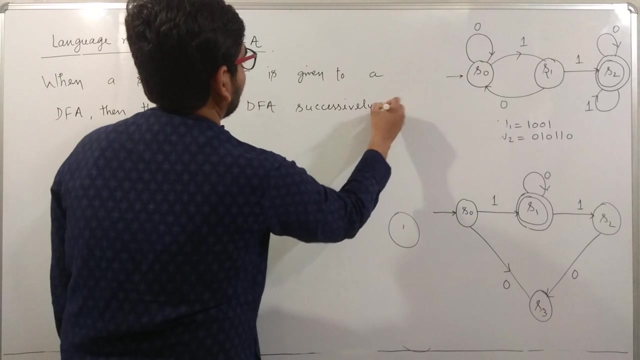 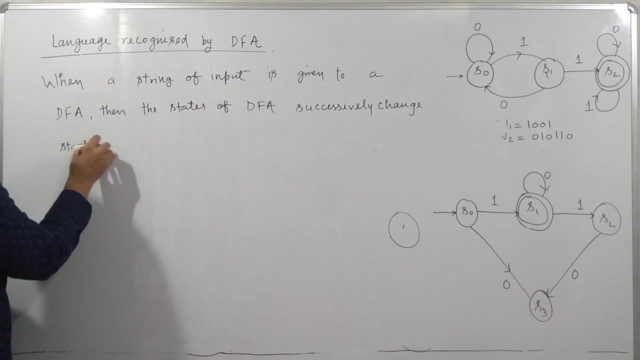 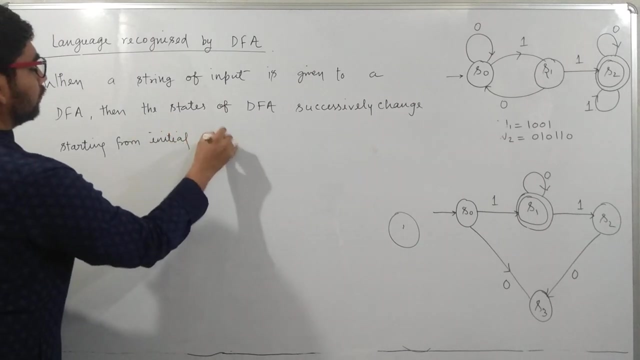 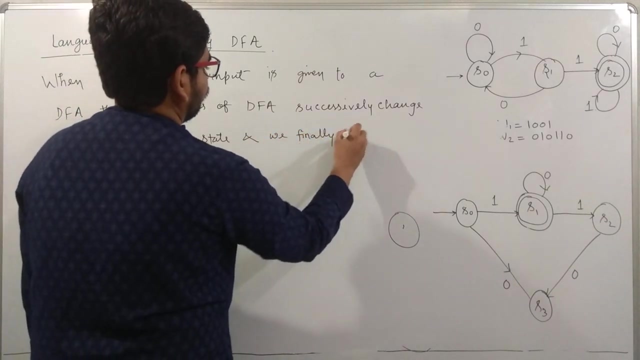 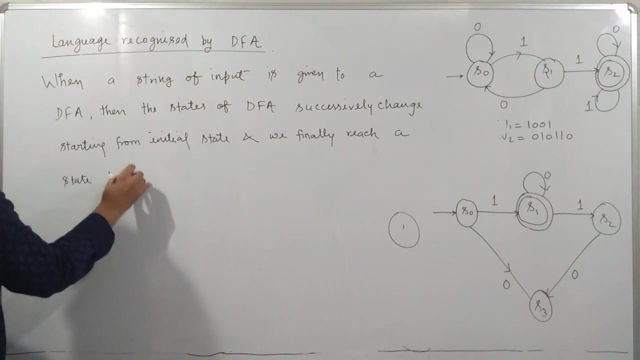 or this type of string is accepting The language recognized by DFA. we can see the definition of this: when a string of input is given to a DFA, then the states of DFA successively, successively change, starting from initial state, and we finally reach a state by the. 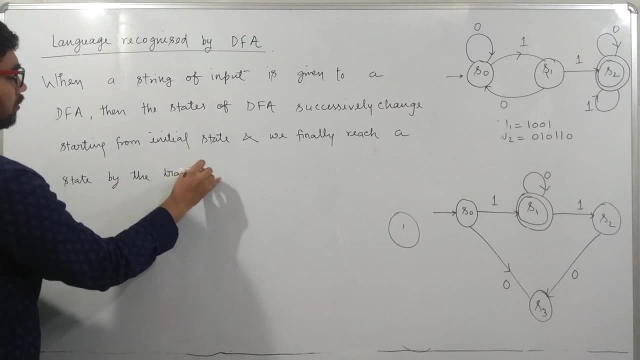 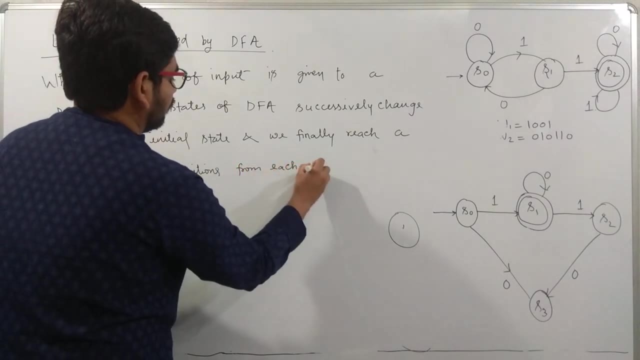 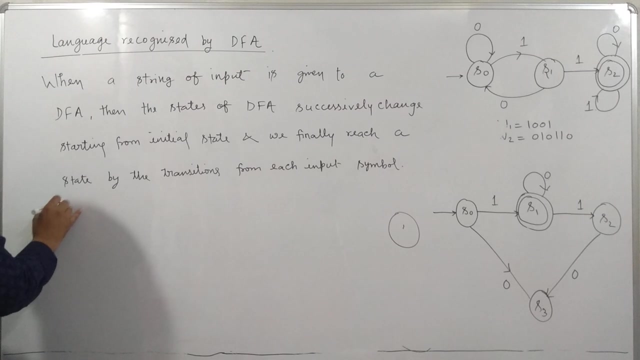 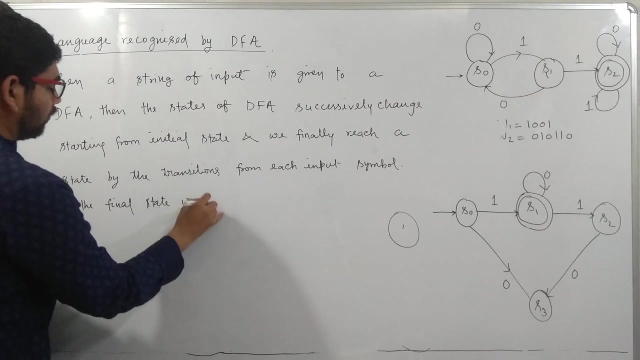 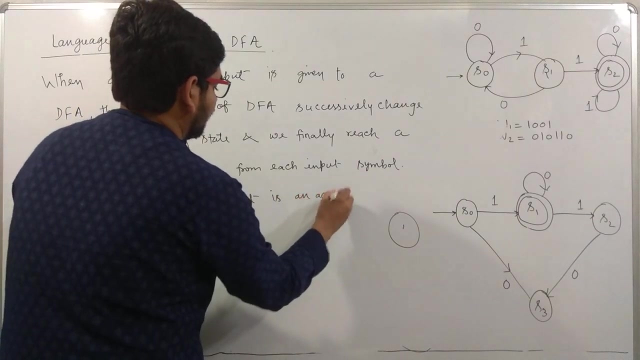 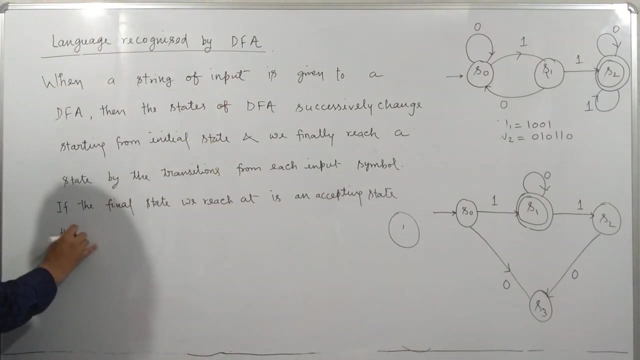 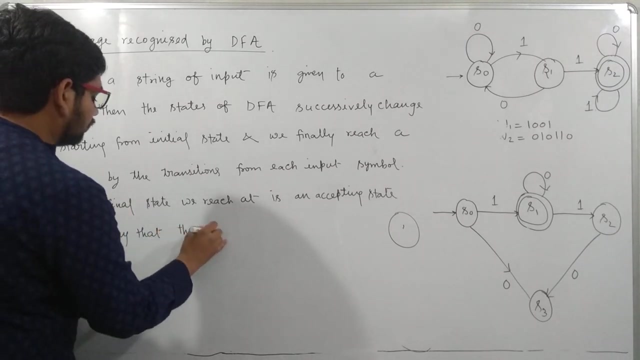 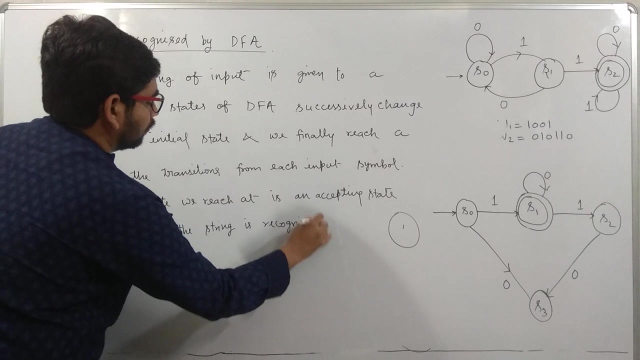 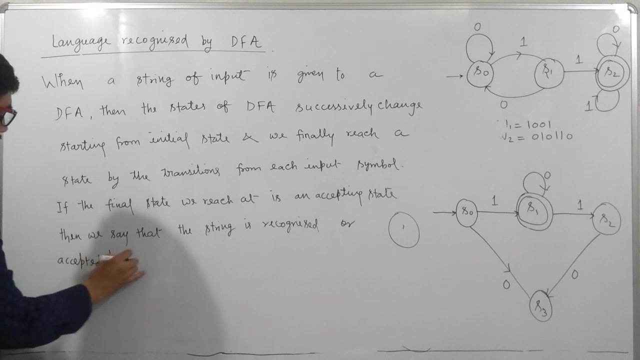 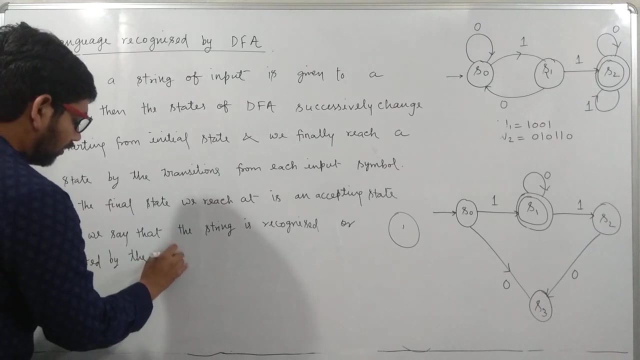 transitions from each input symbol. if the final state we reach at is an accepting state, then we say that. then we say that the string is recognized. string is recognized or accepted by the. the string is recognized or accepted by the DFA. string is recognized and accepted by the DFA. 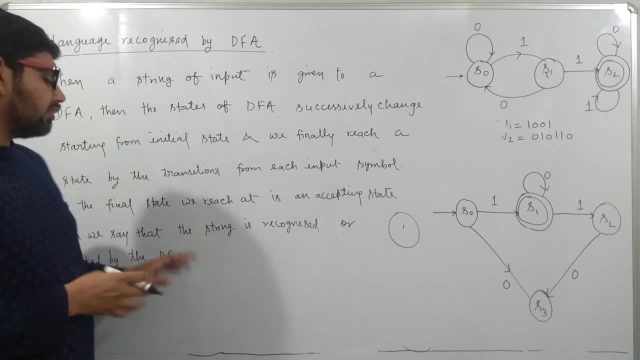 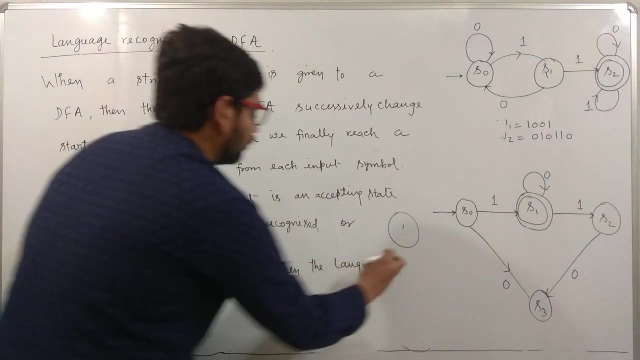 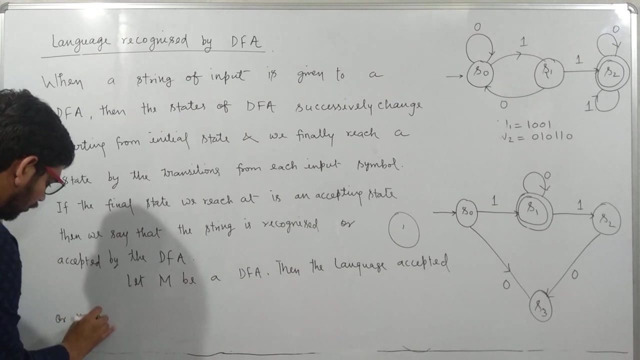 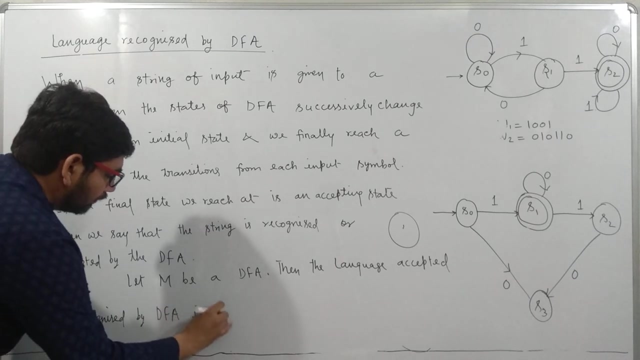 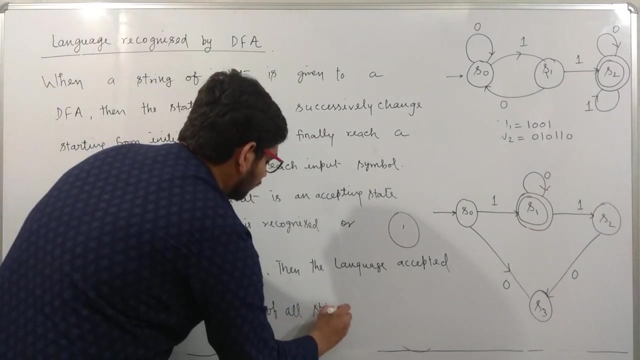 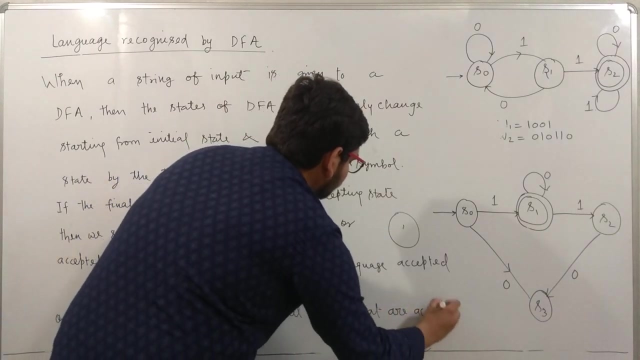 so if the final state that we are getting is an accepting state, then we say: the string is recognized or accepted by the DFA- let M be DFA. then the language accepted or recognized by DFA is the set of all strings, is the set of all strings that are accepted by. 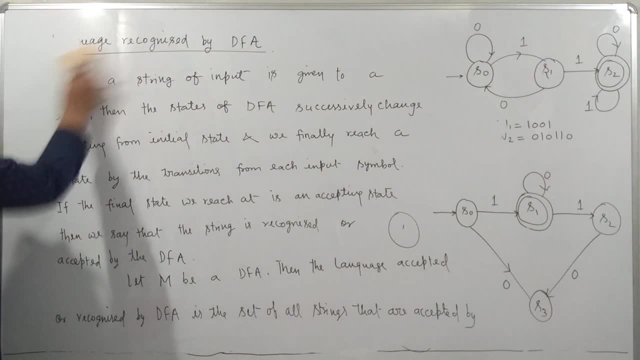 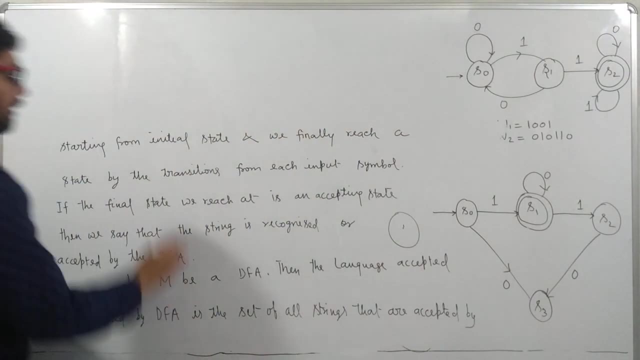 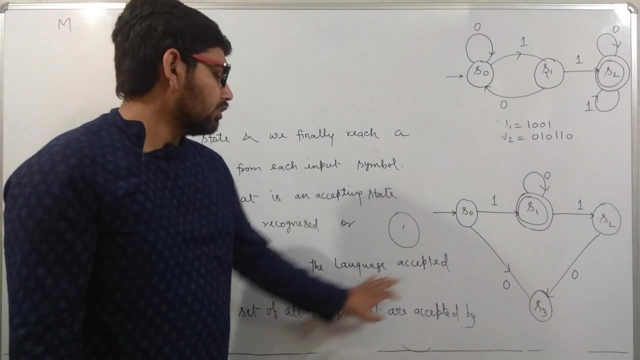 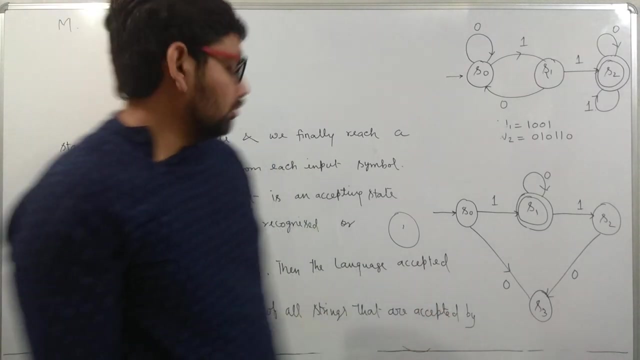 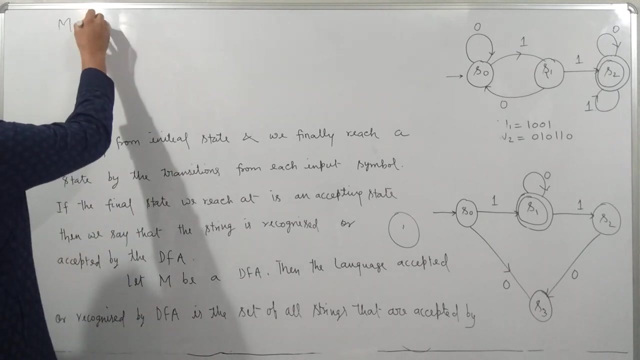 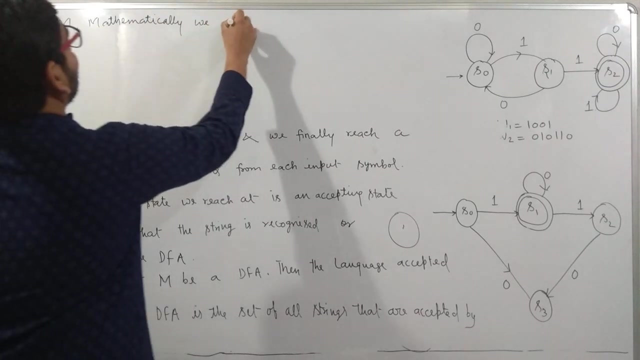 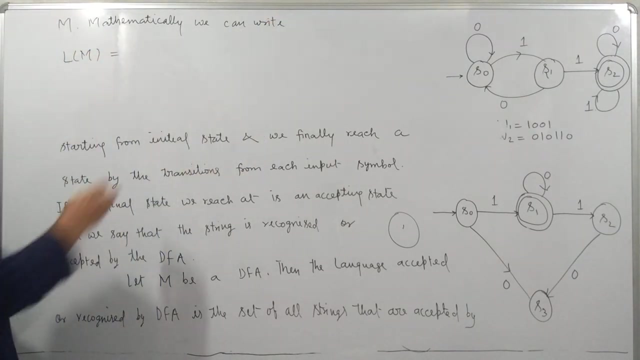 by, by by, that are accepted by M, that are accepted by M. So the language accepted or recognized by DFA is the set of all strings that are accepted by M, that are accepted by M, that are accepted by M Mathematically. Mathematically we can write: Lm is a language accepted by M. 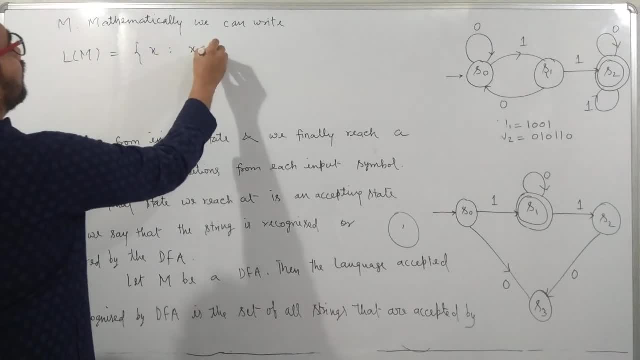 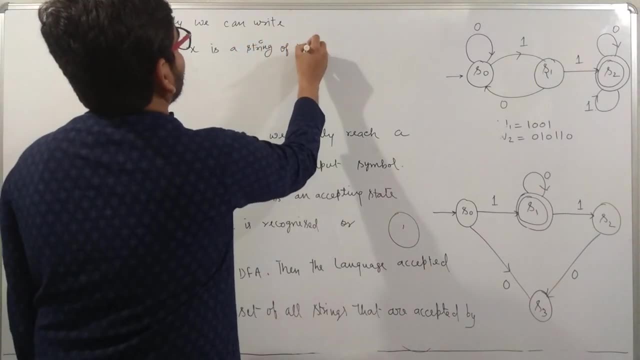 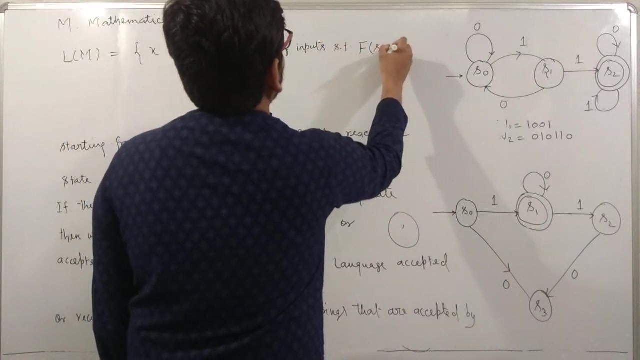 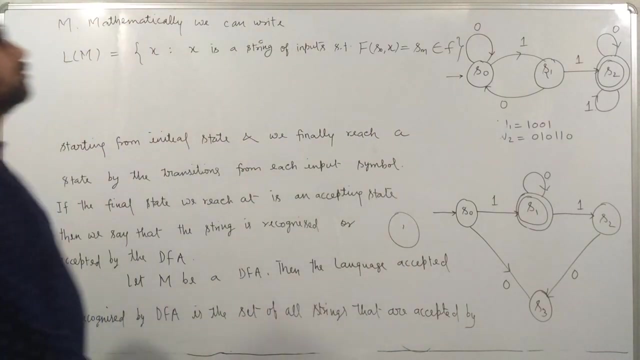 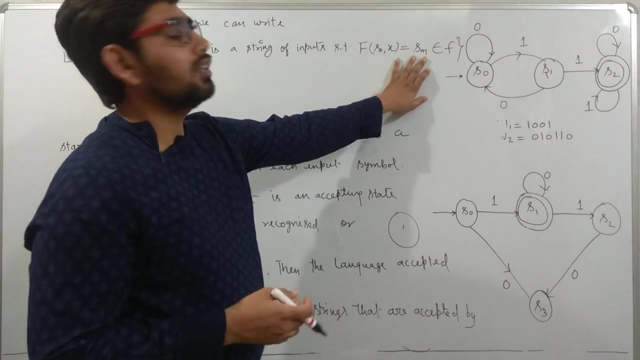 It has x type of elements. x is a string of inputs such that f, when operated on x, gives state sm, which belongs to f. When we apply x string from s0 starting state, then the state we have, the final state, belongs to f. 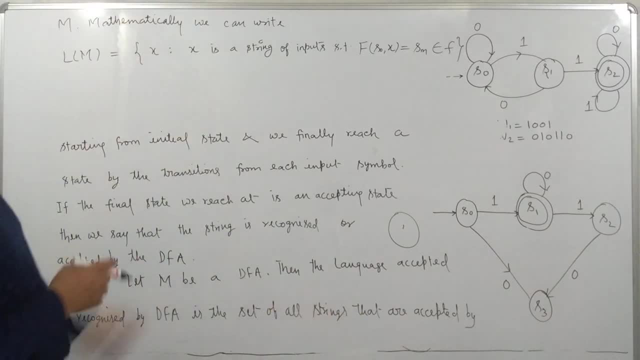 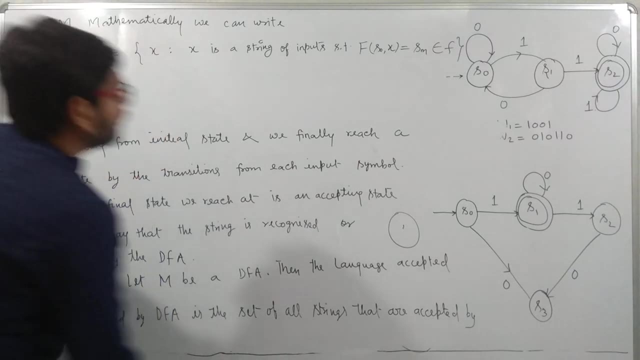 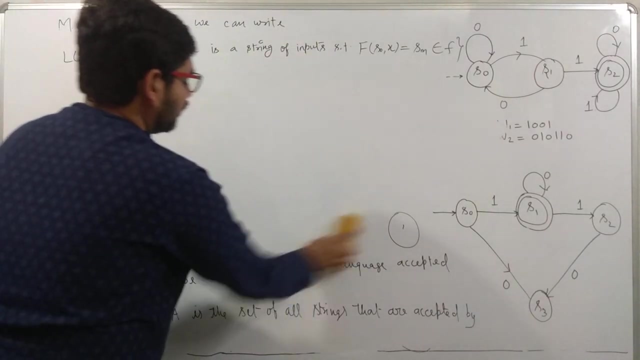 This is accepting state, So we will say that x will be its element, otherwise x will not be its element. This is the definition of language: A state in which we get trapped, in which there is no accepting state. and if we reach there, 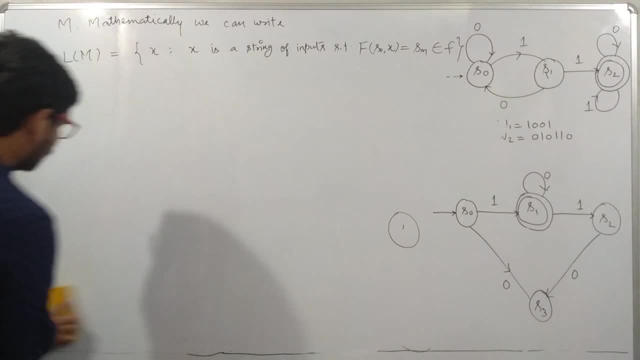 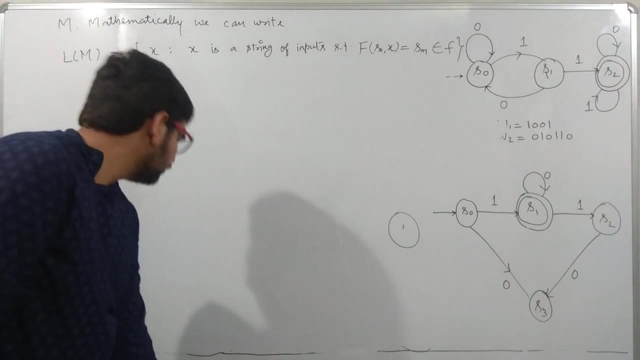 then we cannot get out of it. Such a state is called trapped state and dead state. Trapped state and dead state. Now I will show you two questions. These two questions will be done one by one. First, let's come to the first question. 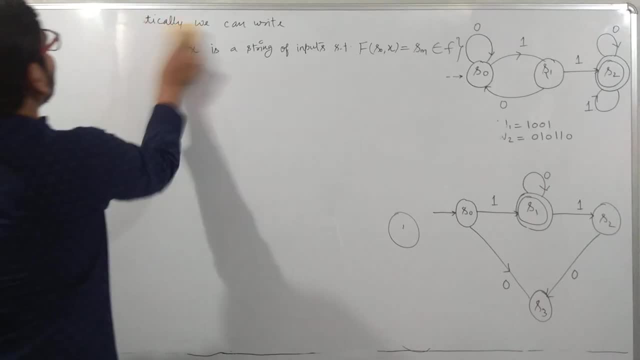 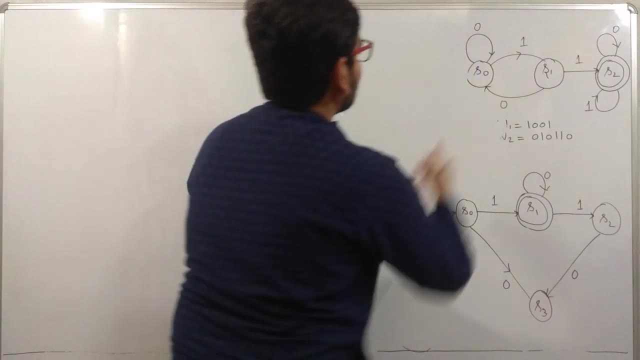 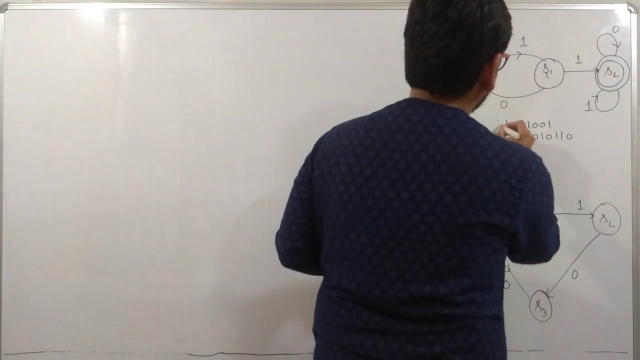 Let me paste the definition. See what is the first question. In the first question we have given a transition diagram. This is the first question we have. This is a transition diagram. There are three states in it: s0, s1, s2.. 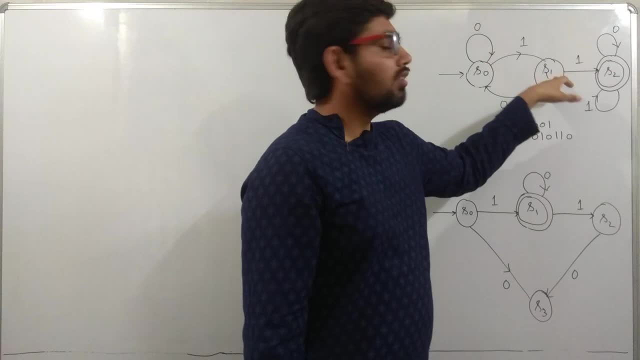 s0 is given as 0, s0 is given as 1, s1 is given as 1.. Transition has taken place. We have read this before. s2 is the accepting state here. What do we have to find first? 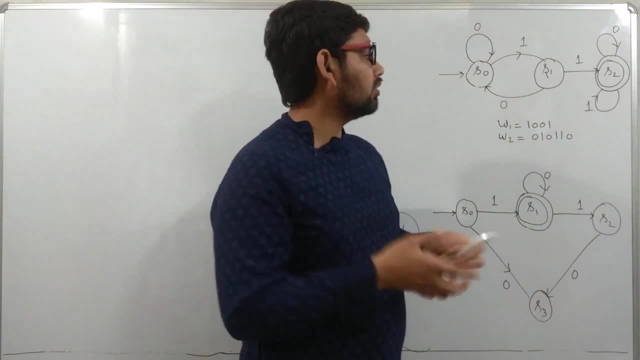 First 1001.. This is the string. When we update this string on it, then what state will we get? We have to find that W2, we have to find that. Then we will tell it that W1 and W2, these strings. 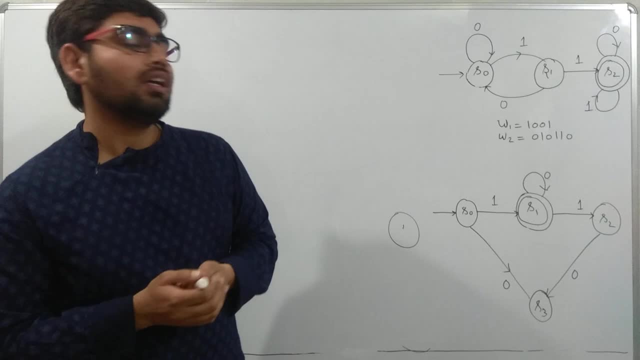 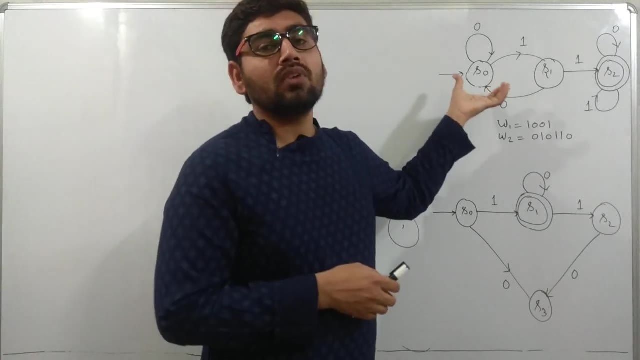 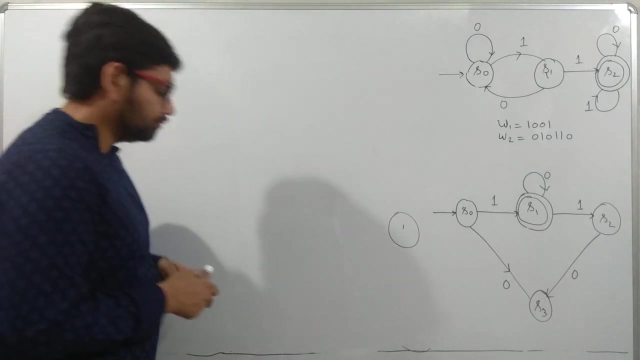 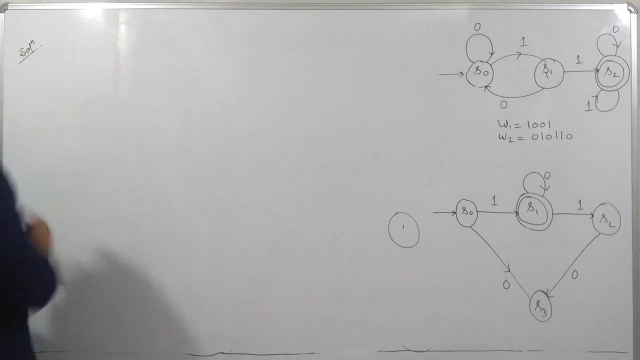 are they being accepted or not? And when they are being accepted or not, then we will decide that which type of language will this machine accept or recognize? This deterministic finite state automator will recognize which type of language. So we will do it in three parts. 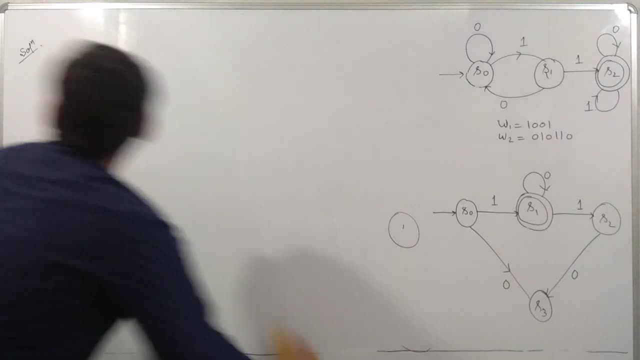 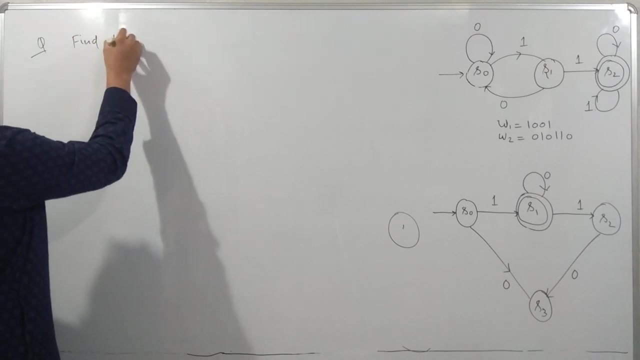 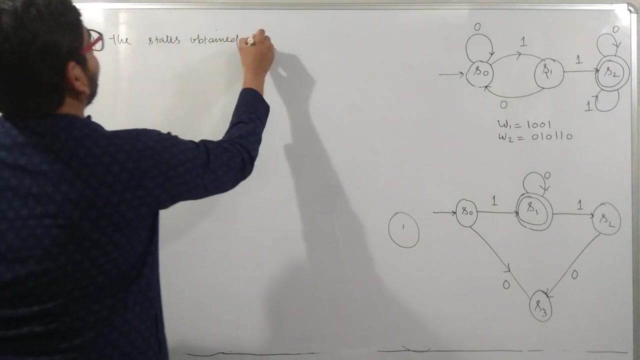 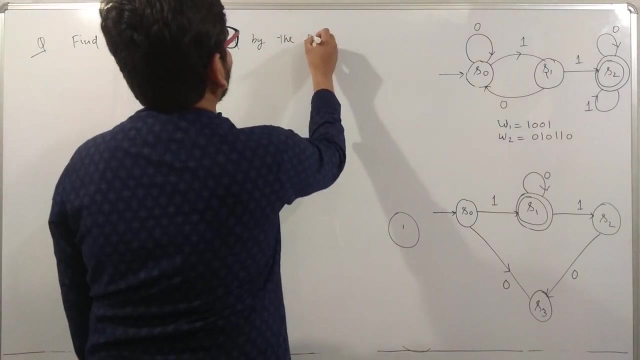 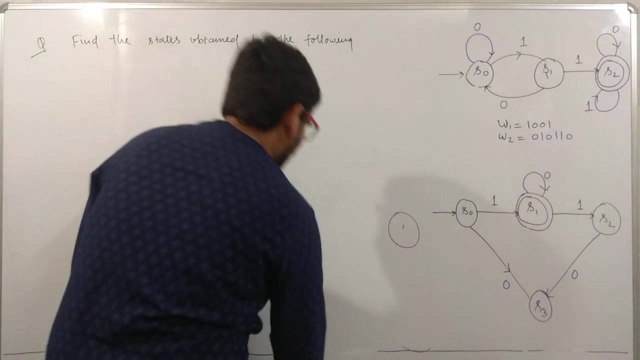 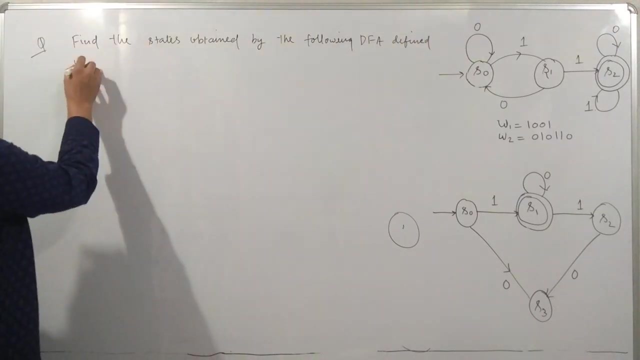 If you want to write a question, then note down the question first. Find the states obtained by the following DFE: Find the states obtained by the following DFE: This is defined by a state diagram. This is defined by the following DFE: 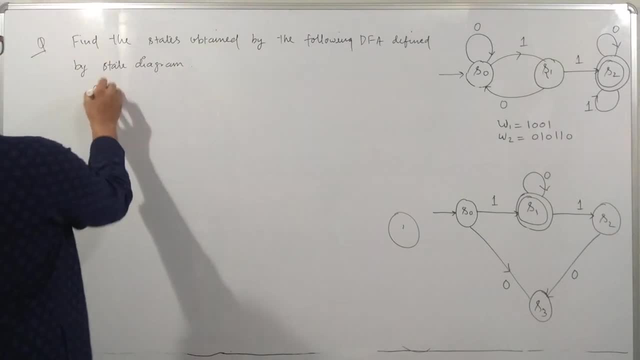 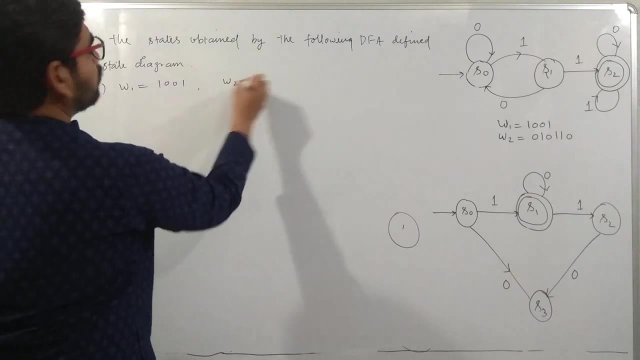 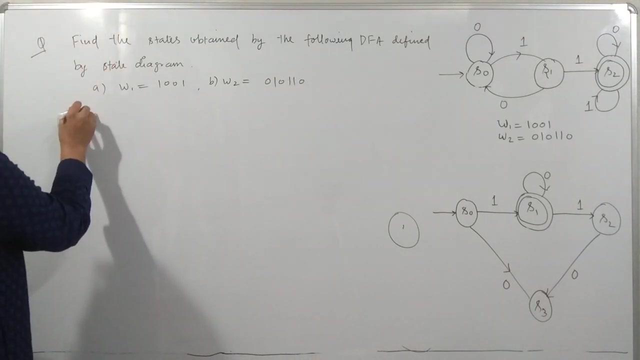 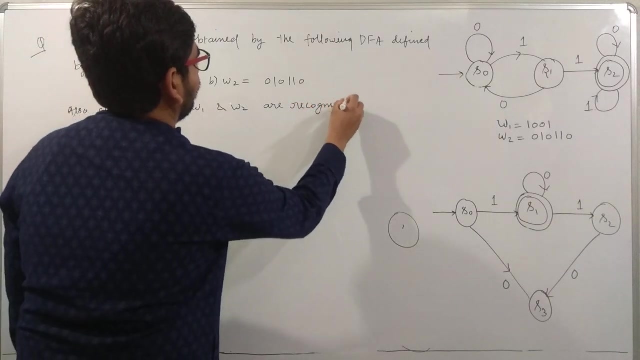 This is defined by the state diagram. A is: W1 equals to 1001.. This is the corresponding finite term. W2 equals to 010110.. This is the corresponding. also also check whether w1 and w2 are recognized by DFA or not. 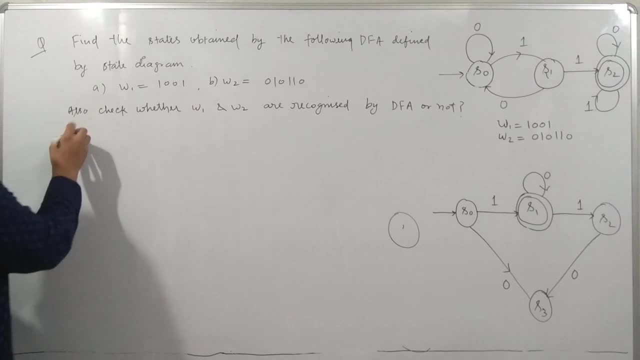 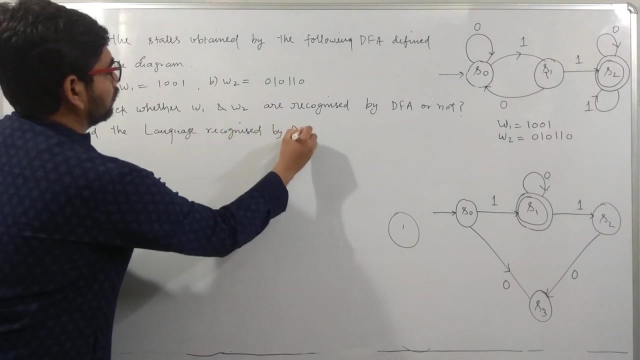 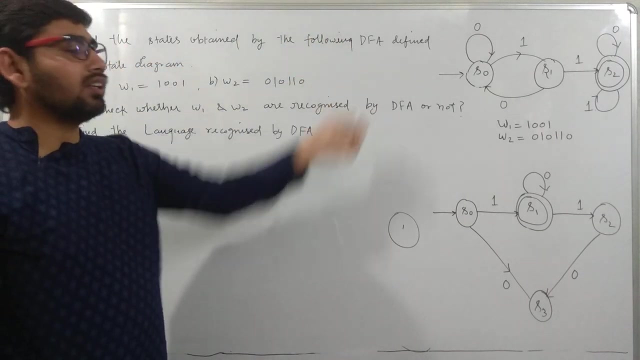 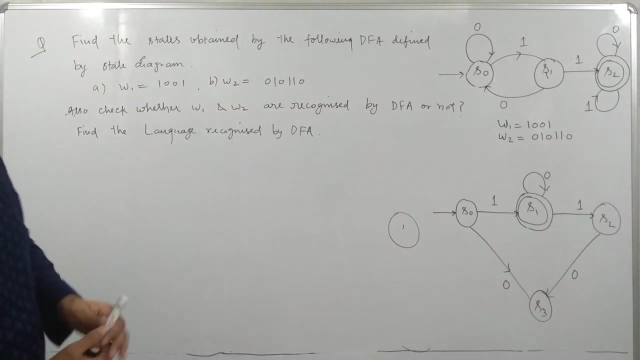 find the language recognized by DFA. these are the three parts of the question. in the first part, we have to find the corresponding of the following DFA, which is defined in the transition diagram. we will give the input of these strings, in which state we will get the input. 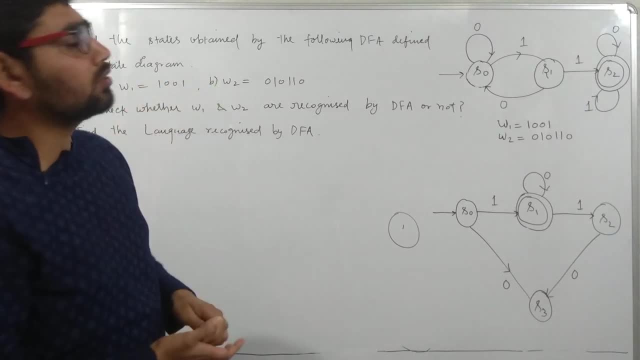 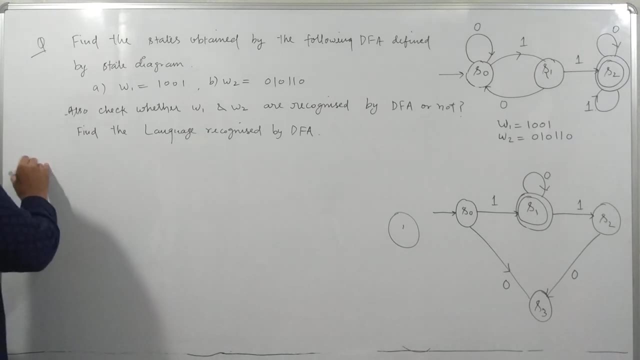 first we have to tell which string is recognized by DFA and in the third we have to tell which language is recognized by DFA. for that, for the first part, we have to take w1 input. we will apply w1 string f. the starting state is s0. 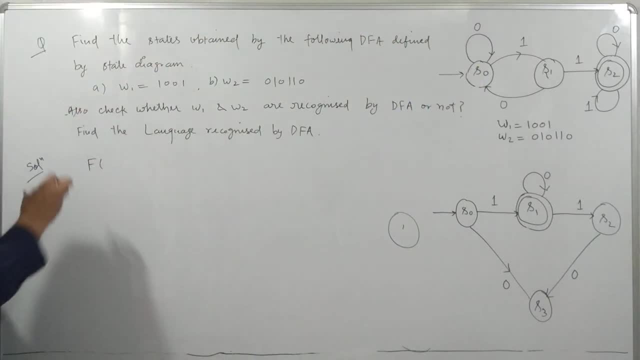 we will give the input of s0 first. we are doing a part f, we want s0 and first of all we want to give w1 input. when we give w1 input, string is given which state we will get. we have to find this. 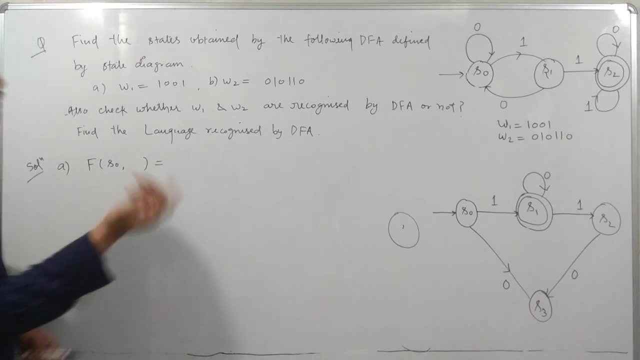 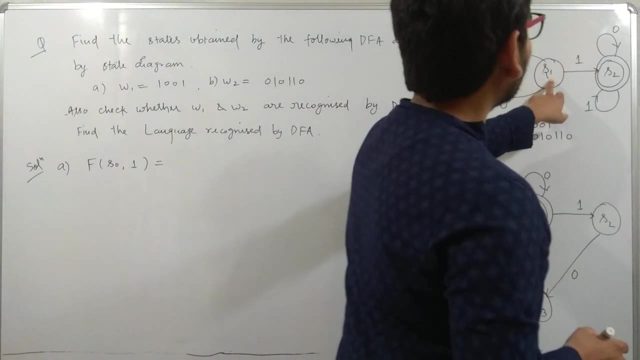 for this. we will not give w1 input. we will apply w1's first input symbol, 1. when we give 1 input, f, s0 1, 2. when we give s0 1 input, we are in s1 state according to the transition diagram. 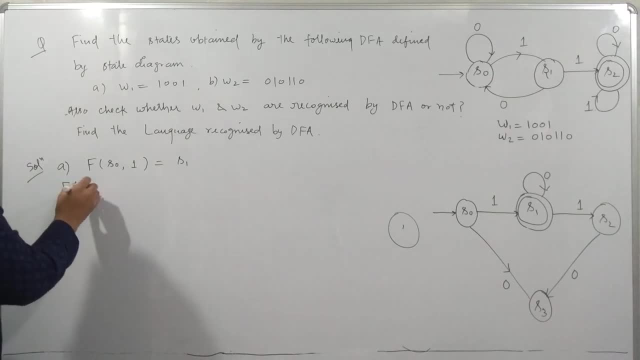 we will get s1. now what will happen in the next step? in the next step, what will happen when we give w1 input? now we will give w1 and 0, that is, we will give the entire string w1- 0. 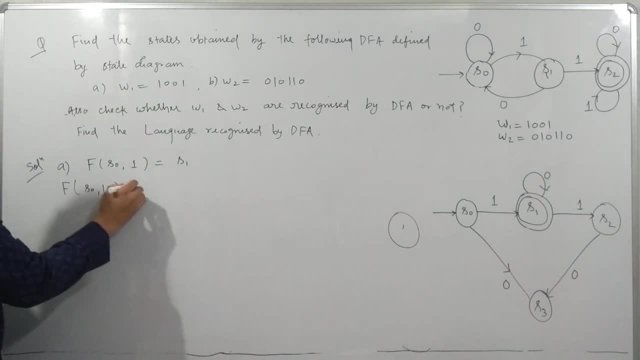 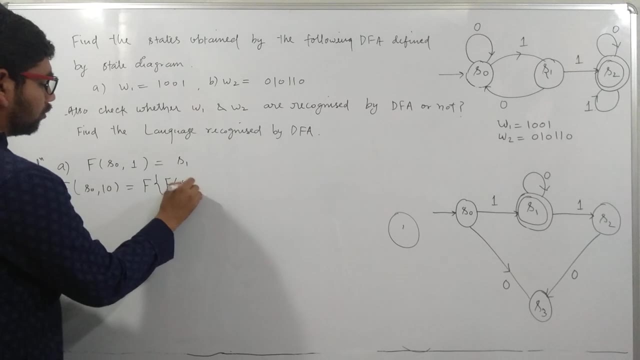 we want to find the corresponding of w1: 0. to find the corresponding of w1: 0. we have already found. we will write like this: we have already given w1 to s0, so the state we got on w1. now what will give the next state? 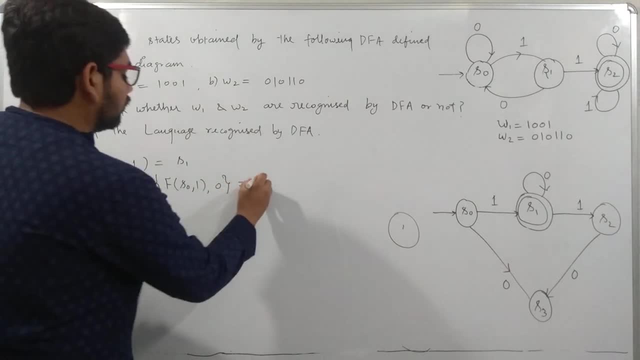 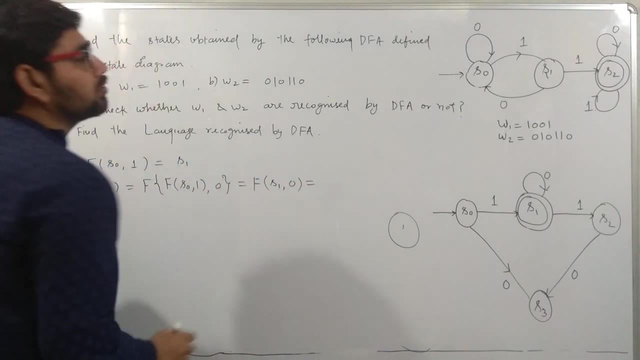 0. we will find it like this: f- we have already found this- f. s0, 1, 2 is s1. we have to give 0 input to s1. we have to give 0 input to s1. so where will we come? we will come to s0. 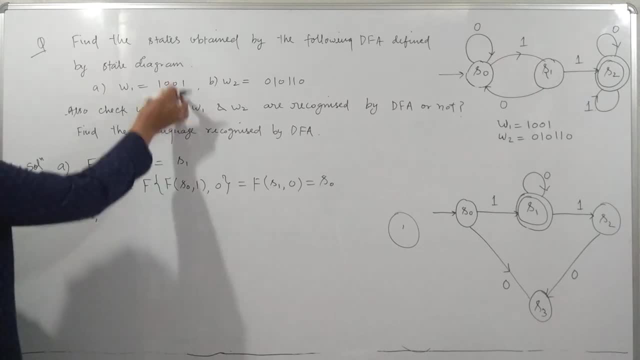 in the same way when we gave s0 1 0. now another symbol has come in the string 0. we have to find the corresponding of 1 0 0, so the corresponding of 1 0 0. we will know the value of s0 1 0. 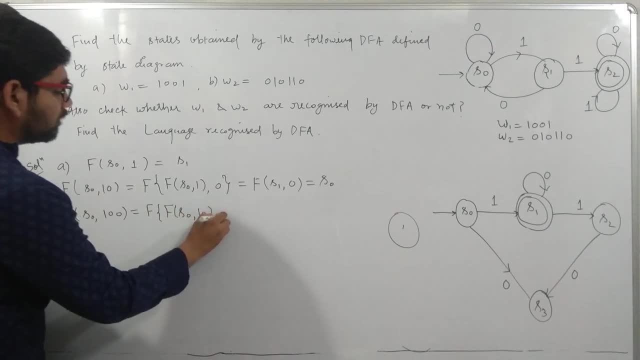 we will apply this first: s0 to 1: 0. whatever state we will get, that is, we will reach the previous state. then we have to give the input symbol. what was the input symbol here? 0. we can write it like this: this state came. 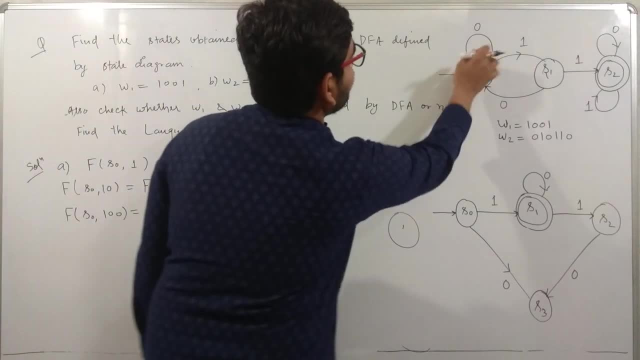 we are giving 0 to s0. if we give 0 to s0, then we will give 0 to s0, we will remain in s0 and finally, we want to give 1 to s0, so we will give 1 to s0. 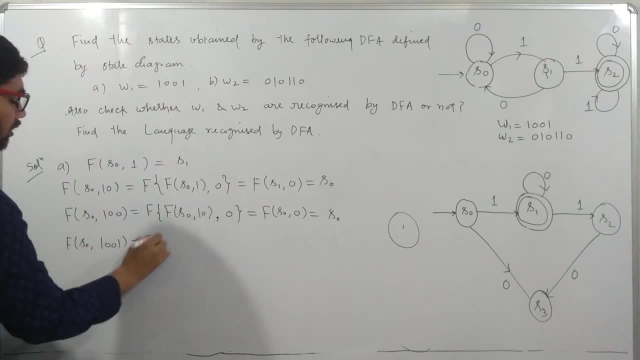 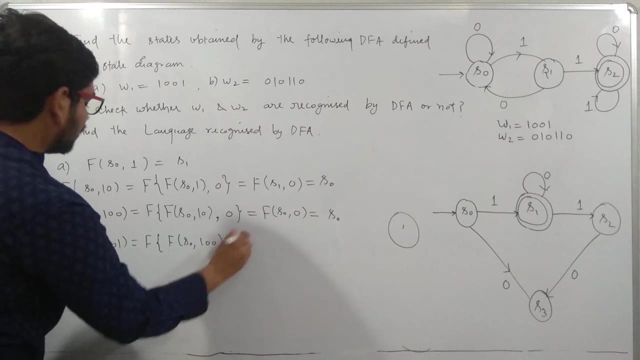 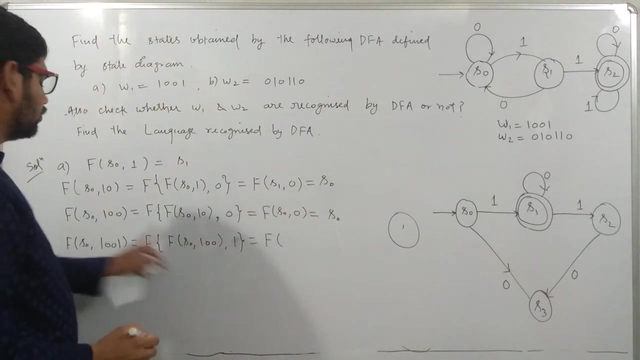 that is the entire string, will be our 1 0 0 1, which means we had given s0 1 0 0 and now we are giving 1. finally, we will give 1. so here, s0 1 0 0. 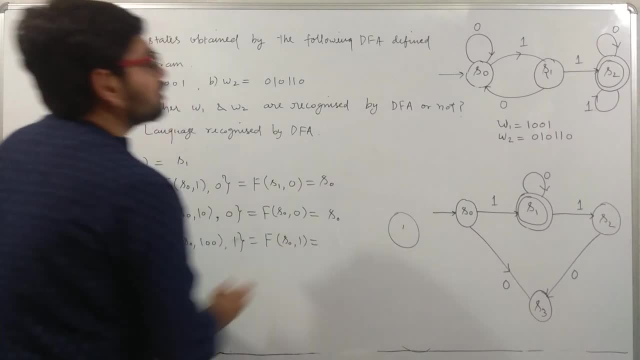 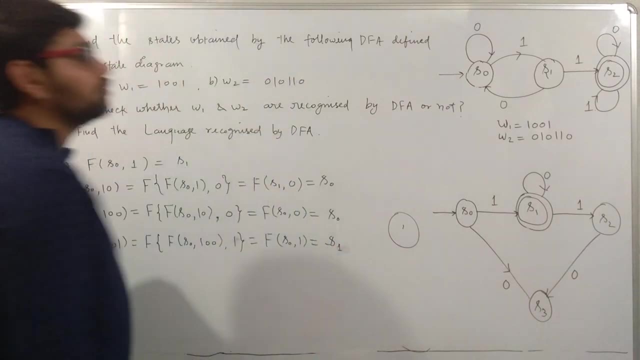 is the first defined s0, we are giving 1 to s0. when we gave 1 to s0, then the state came s1. ok, state s1 came because s1 is not the accepting state. it is defined as 2 only so we can say: 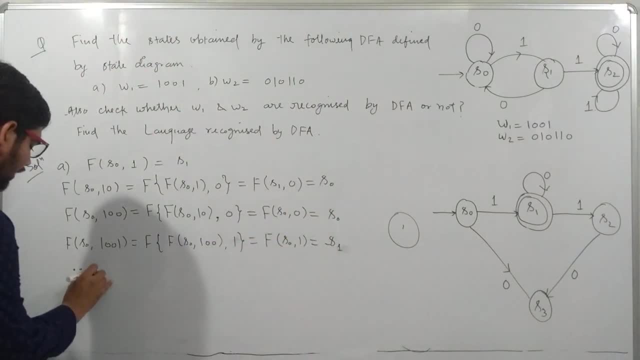 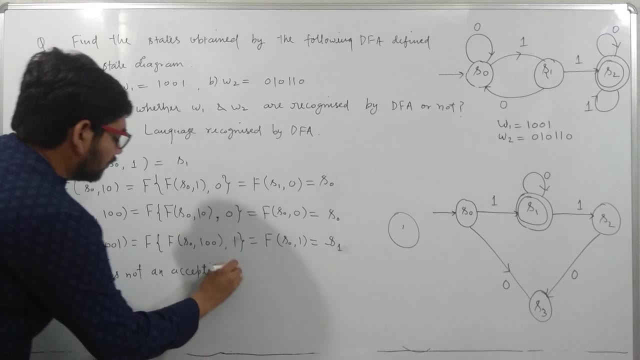 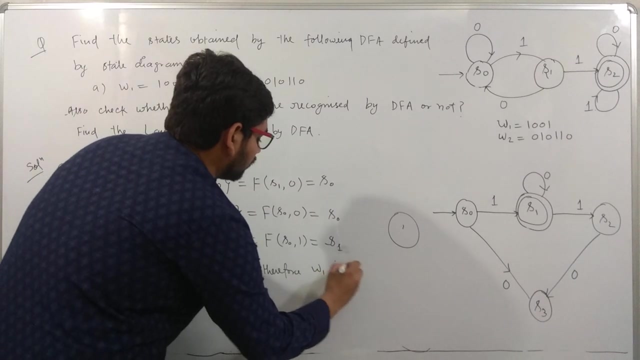 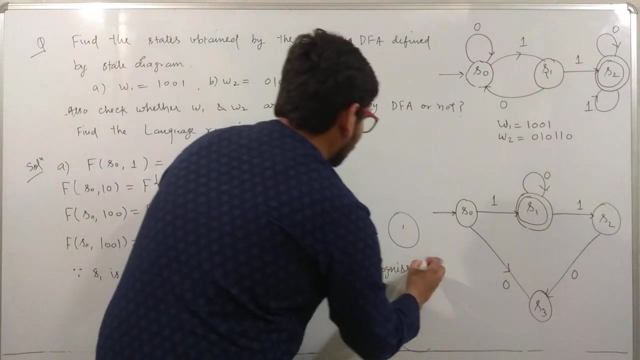 since s1 is not an accepting state. s1 is not an accepting state. therefore, w1 is not recognized. w1 is not recognized. the machine did not recognize this input. w1 is not recognized by DFA. w1 is not recognized by DFA. the machine did not recognize this input. 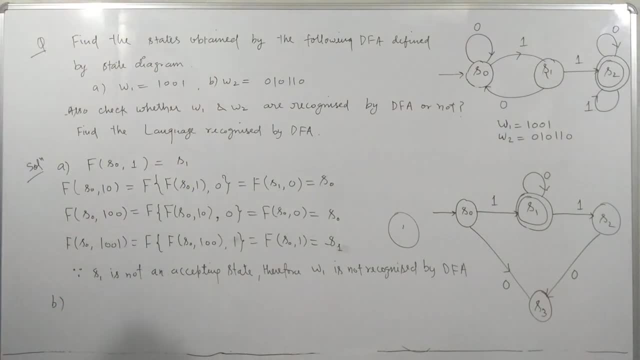 the machine did not recognize this input from DFA. next for w1: we will do. you must have understood this step. I have given an example before. we will do it directly. next: we will do. we will apply directly. we will do f and w2: we will apply. 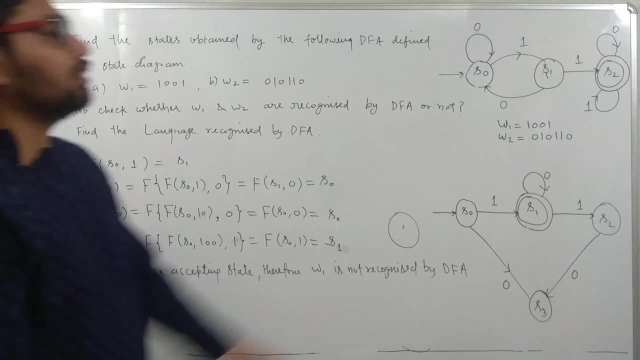 we have applied 0 for w2. we will apply 0, so we will come to which state. we gave 0 to s0, so we will stay in s0. so we will stay in s0, so we will apply s0. 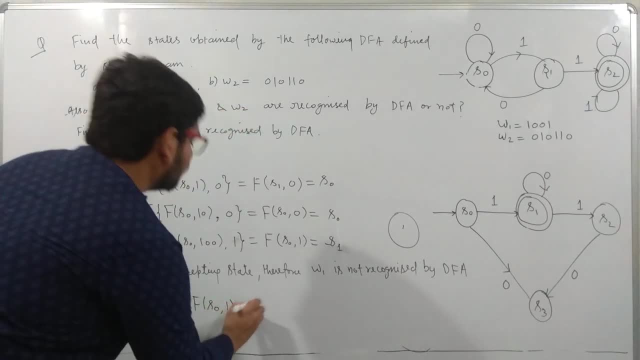 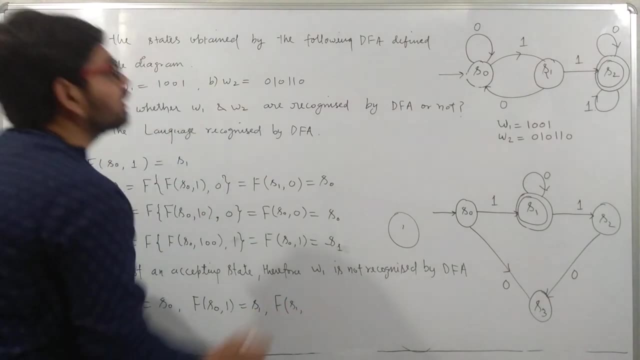 so we will apply s0. next symbol is 1, so we will give 1 to s0. so we give 1 to s1. now we are in s1, so we will start from s1. give input to s1. give 0 to s1. 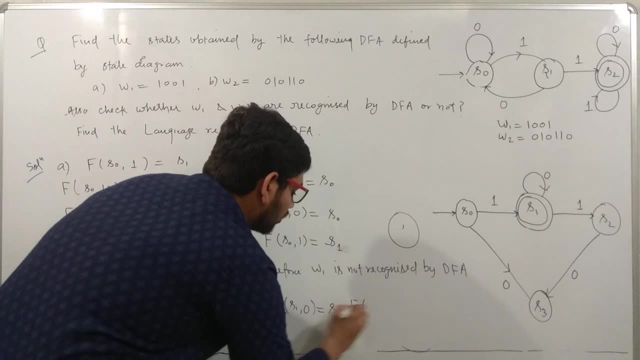 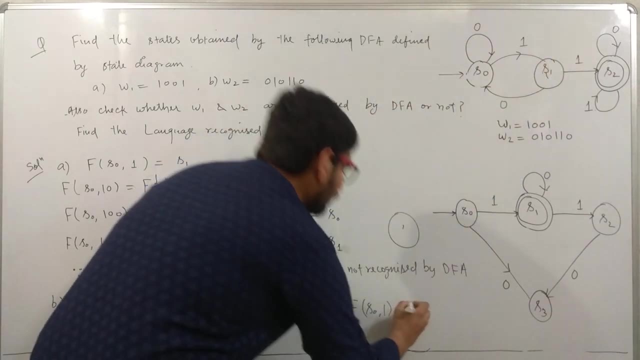 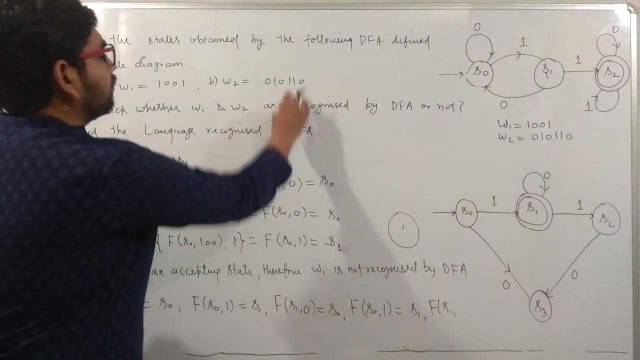 so we are in s0 again. then we will start from where we reached. next symbol is 1. we will give 1 to s0, so we will come to s1. we will come to s1. now we will start from s1. give next symbol to s1. 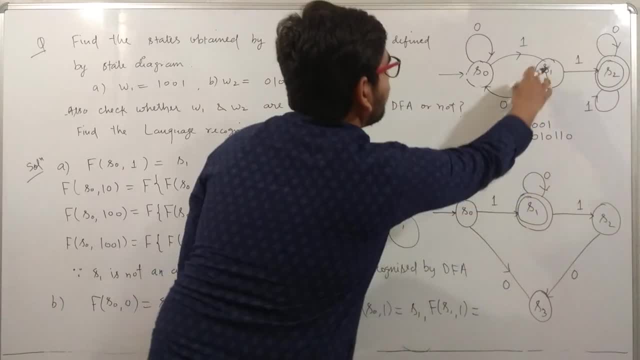 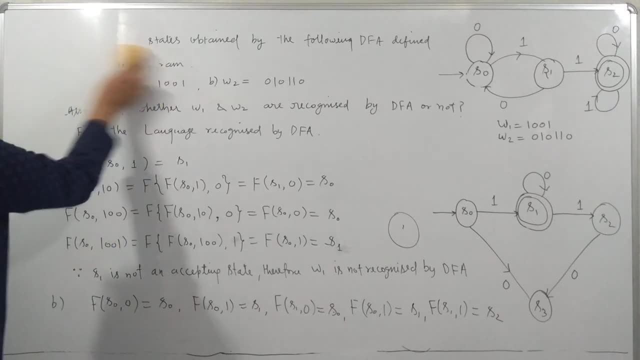 give 1 again. we again give 1 to s1. now we are in s2. now we are giving input to s2. we are giving input to s2. so we are in s2. give 0 to s2. s2 give 0, give 0. 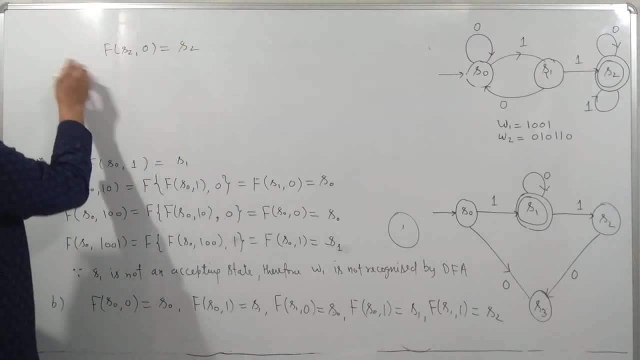 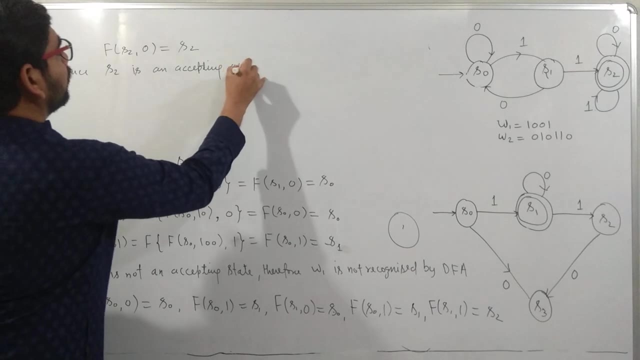 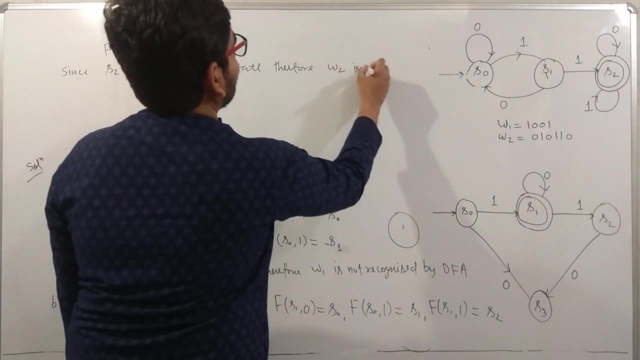 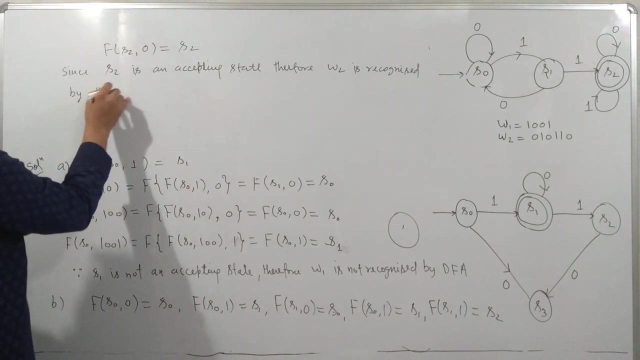 we are in s2, since S2 is an accepting state. Therefore, W2 is recognized. W2 is recognized and accepted by DFA. Now we want to find the language. What we want to find? We want to see what type of strings we have. Which type of strings will be accepted. 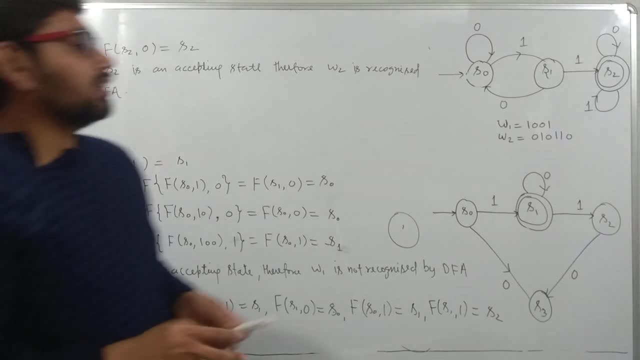 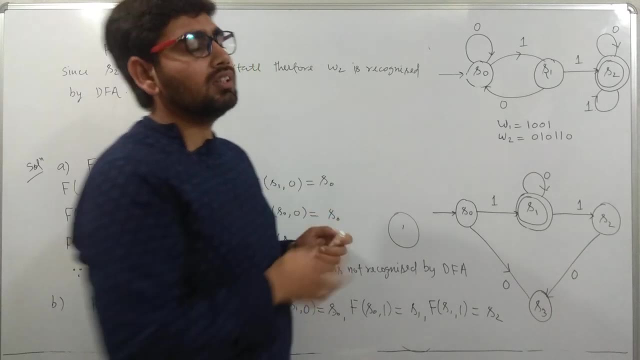 We want to see this. So if you observe here These two types of strings, Let's try to understand this first: 1 0 0, 1. You gave such a string in which 1 0 0, 1 is. This is: 1 is equal to 0 and 0 is equal to 1. 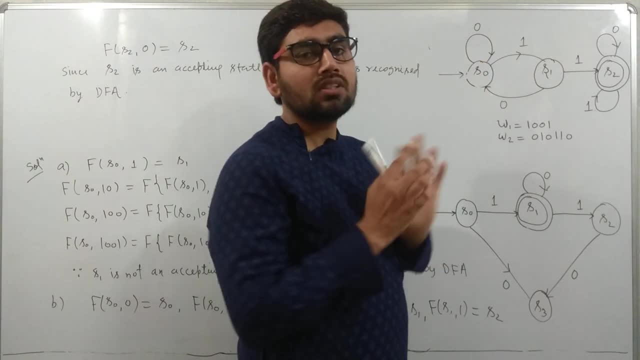 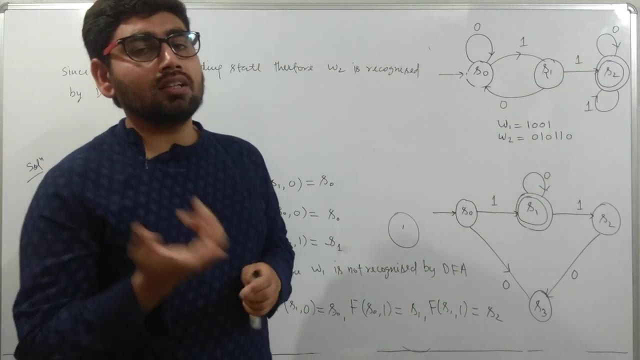 See, if you give 0, then it will remain in the same state. It has to start from S0. And what we want, We want to reach S2 somehow. If we reach S2 Because S2 is an accepting state, There is no way out of S2. 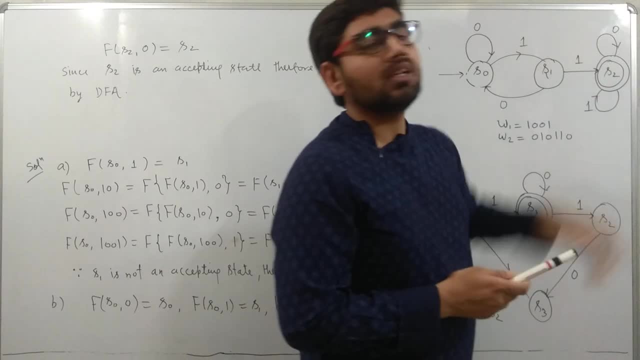 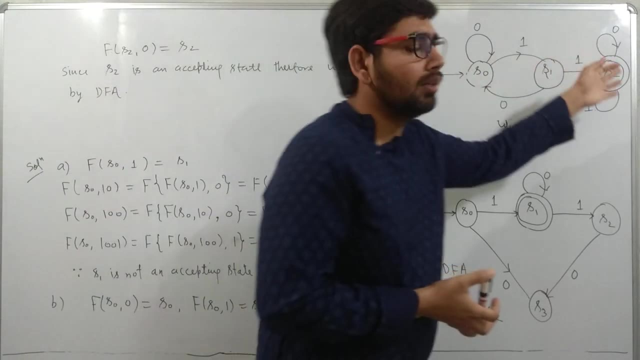 If we give 0, then we will remain in S2. If we give 1, then we will remain in S2. So if we reach S2, S2 is an accepting state, So such strings will be accepted, In which we will reach S2 once. So what will happen to reach S2? 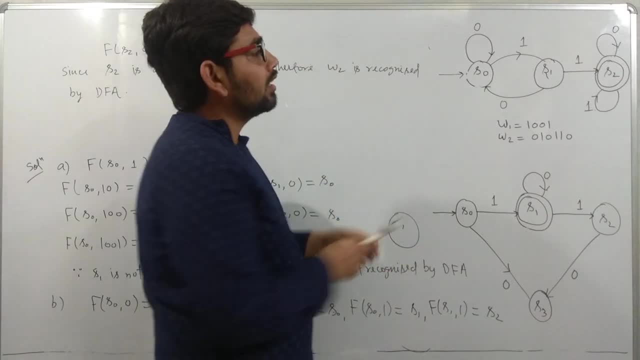 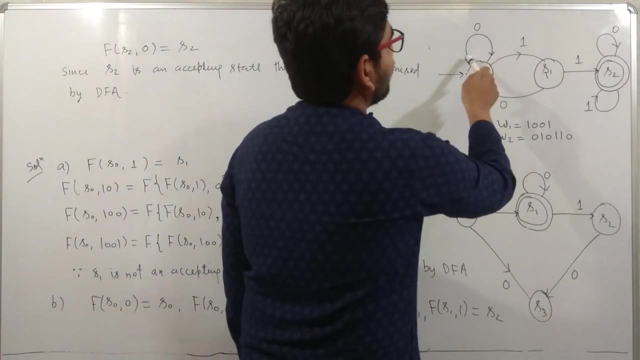 If we give 0, then it does not matter, We stay on it. If we give 1, then we come to S1. If we give 0 to S1, then we come back to S0. If we give 0 to S1, then we come back to S1. 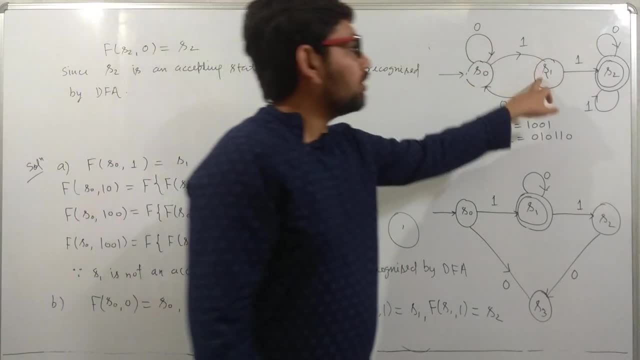 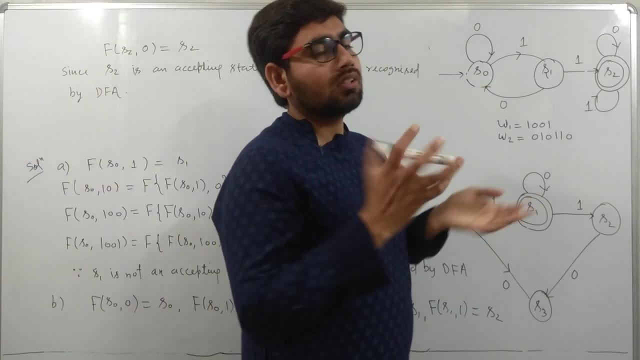 If we give 1, then we come back to S1, But if we reach S1, then we give 1, Then we reach S2. So we are observing here When we start from S0, Because S0 is an accepting state, So whether you give 0 or not, 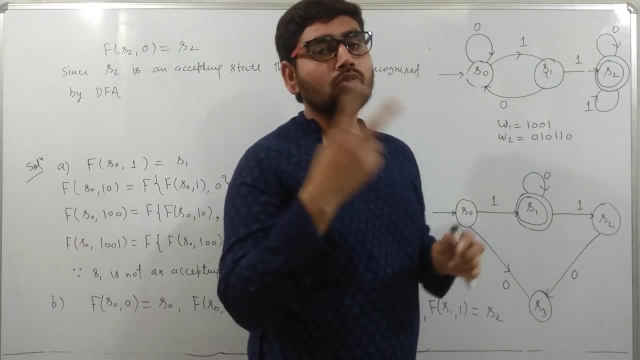 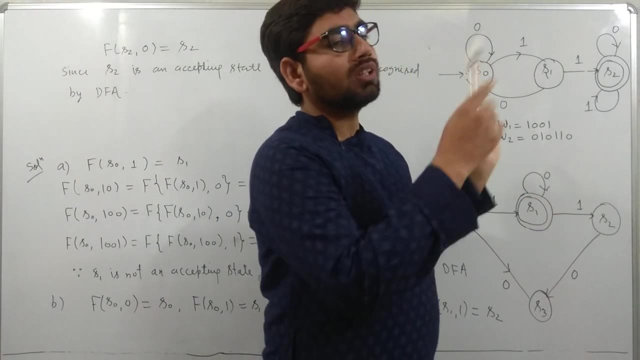 If you give 1 and 1 again Means if you have 2 successive 1, If you have taken such a string In which 2 successive 1 came, No matter how many times 0 has come, How many times 1 has come in the middle. 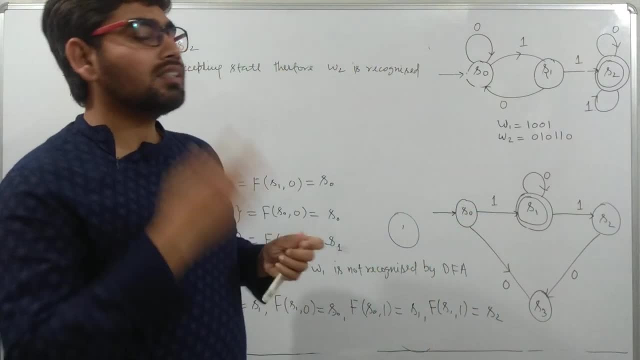 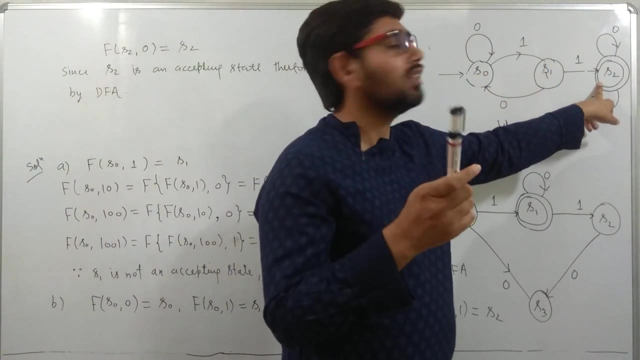 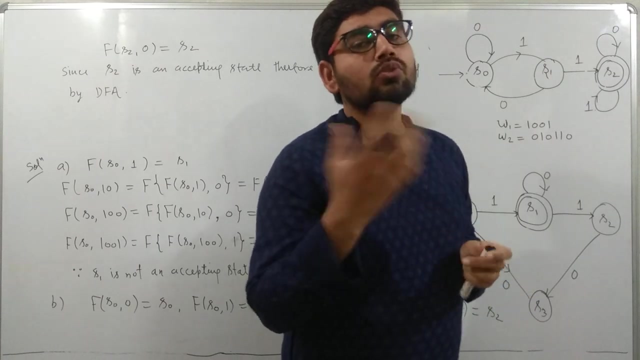 But 2 successive 1, 2 successive 1. In this type of string 2 successive 1 will come Once 1, then 2 times 1 When 2 successive strings come. So we can say We observe that When 2 successive 1 come. 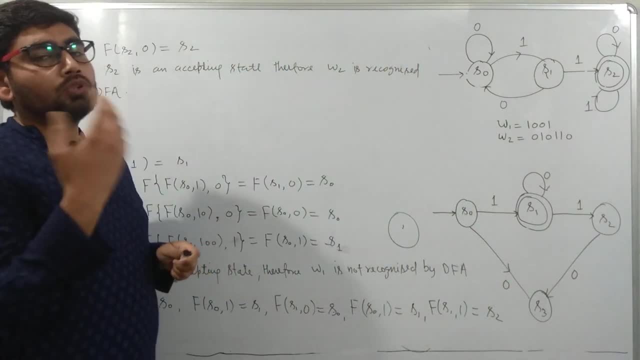 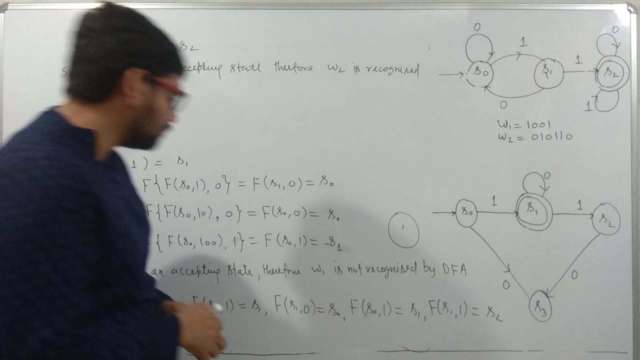 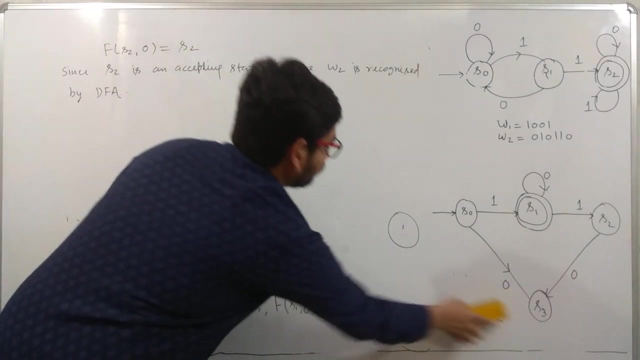 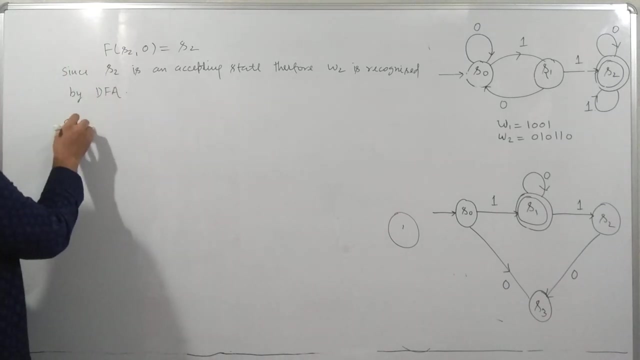 S2 will reach S2 And S2 is an accepting state. If you give 0 or 1, then it will remain in S2 Means our string will be accepted. So what type of language will be accepted? The language of such strings We will define, Since 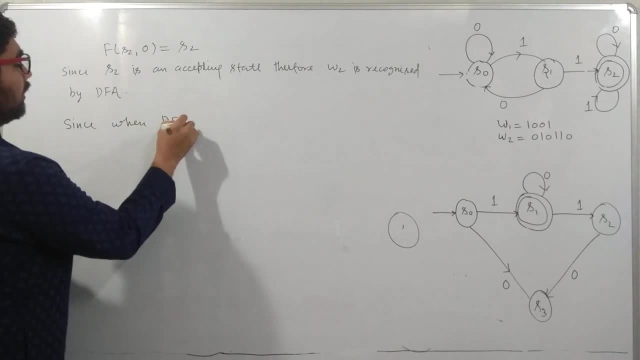 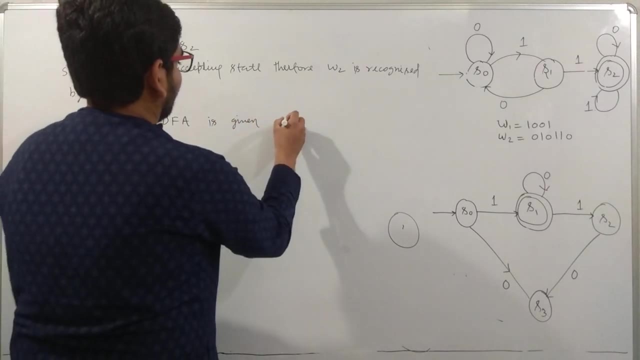 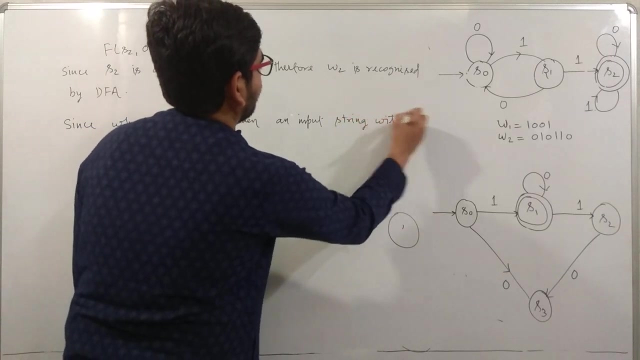 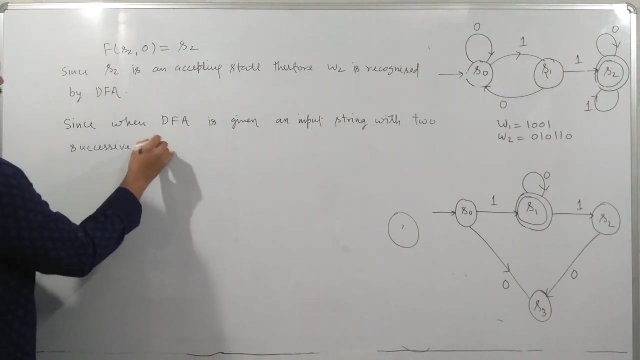 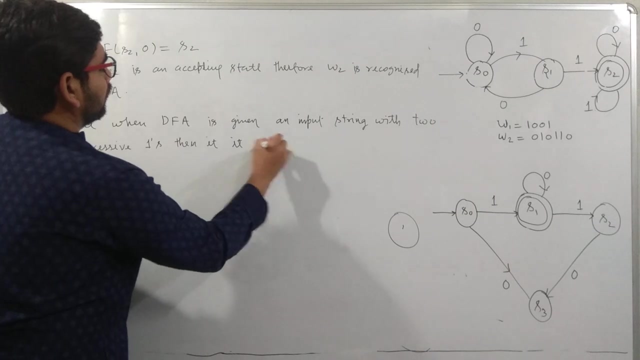 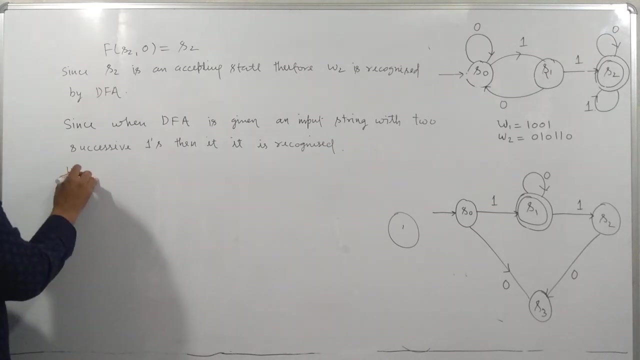 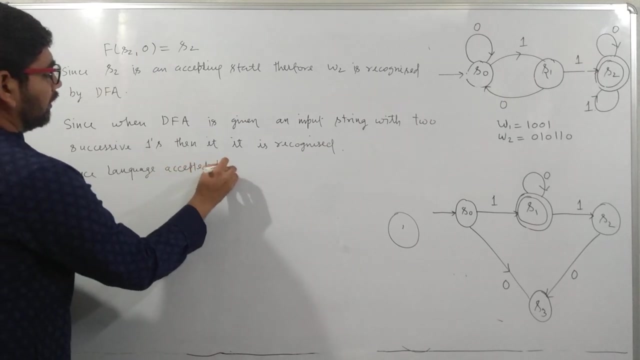 When DFA Is given An input string With 2 successive 1s, With 2 successive 1s, With 2 successive 1s, Then Then It Is Recognized, Then It is recognized. Hence Language Accepted By DFA. Which language is being accepted? It will have elements of x type. 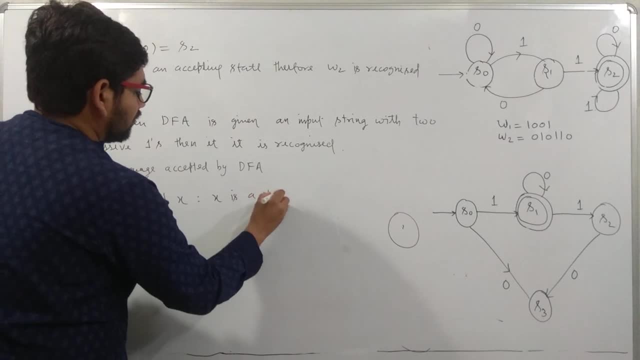 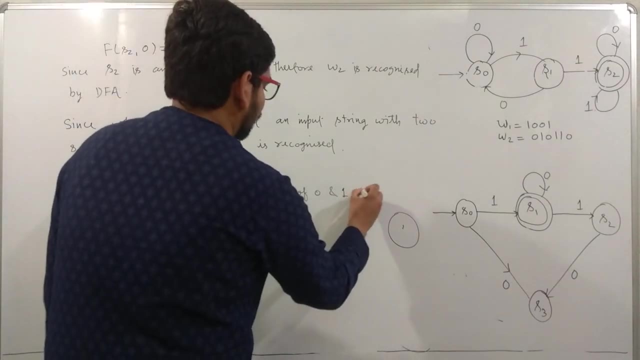 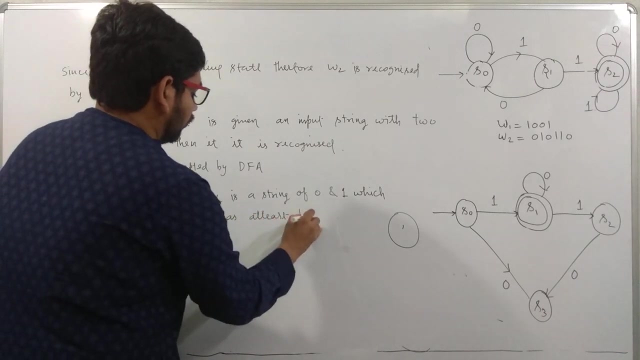 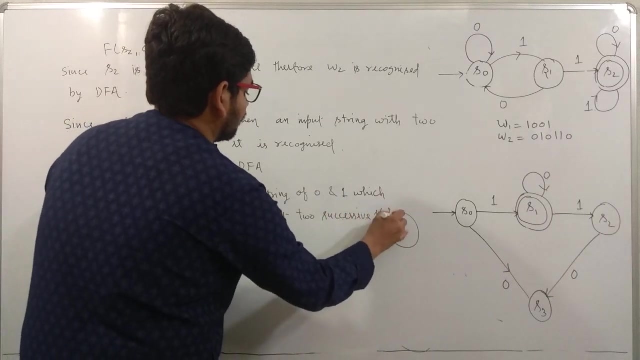 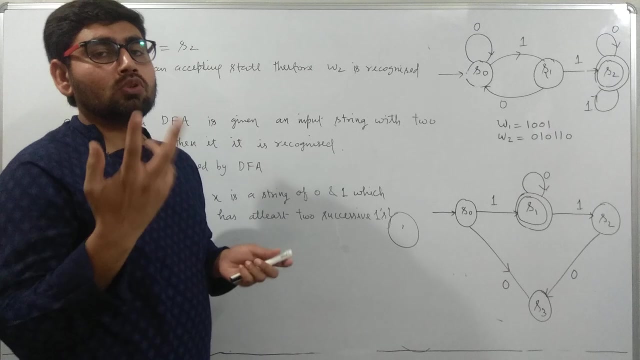 Such that X is a string Of 0 and 1, 0 and 1, Which has, Which has At least At least 2 Successive 1s, Which has At least 2 successive 1s. Such a string, 0 and 1, Which has at least 2 successive 1s. 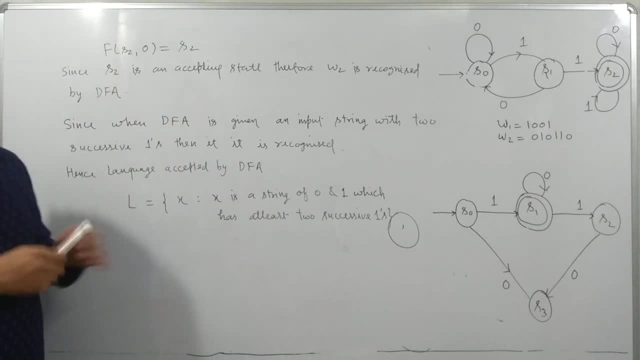 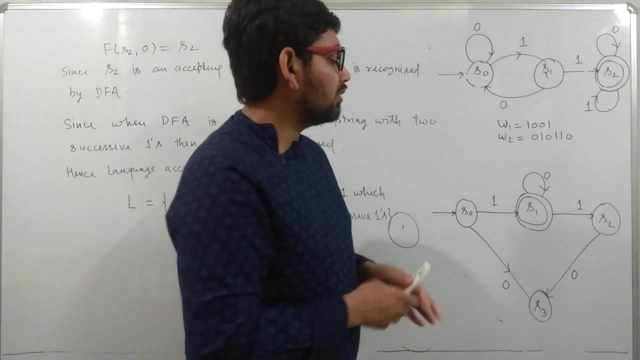 Which has at least 2 successive 1s. These types of strings will be accepted, And the language that is being accepted is Lj. Here we can define it like this. So this question is complete. Let's come to the next question. In the next question we have to find the language. 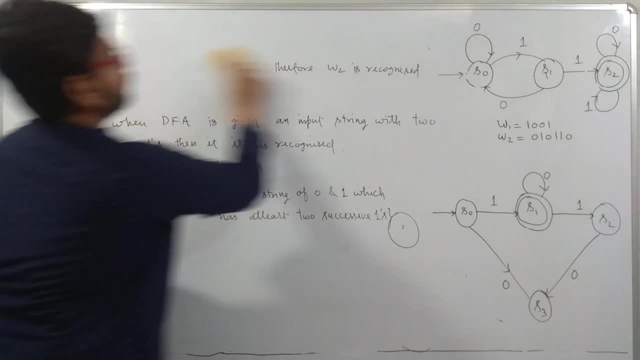 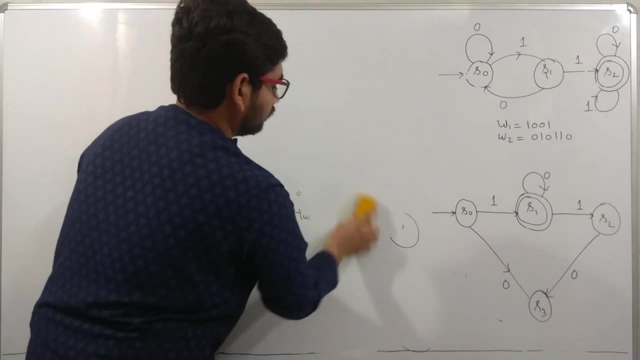 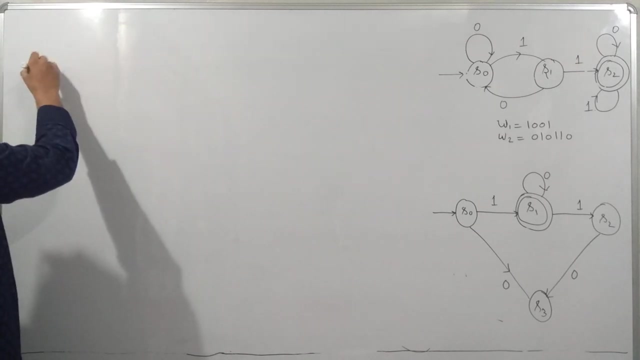 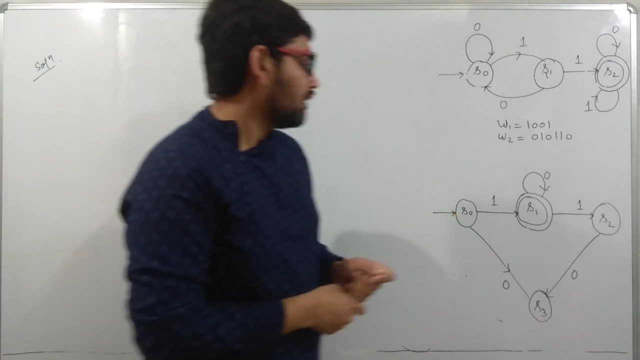 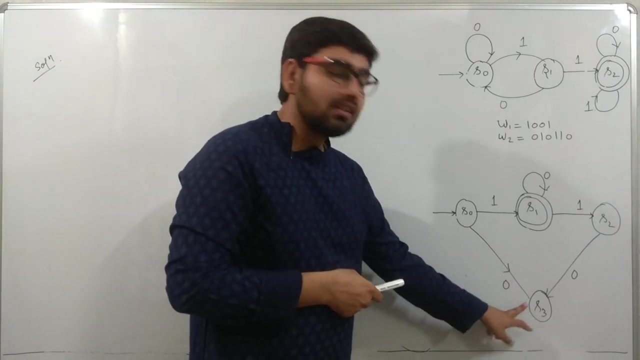 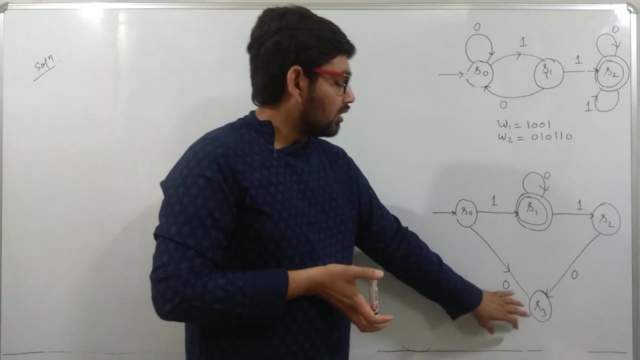 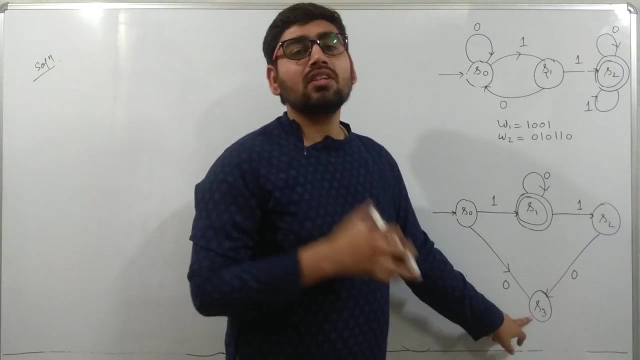 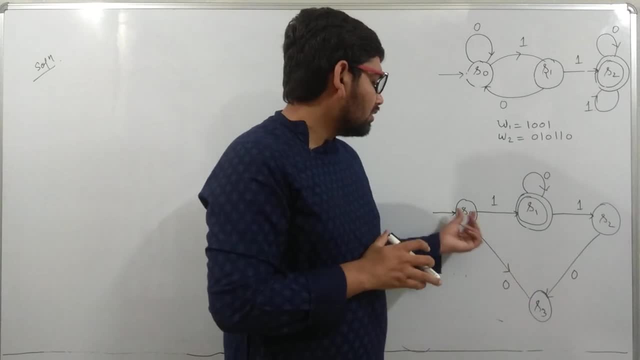 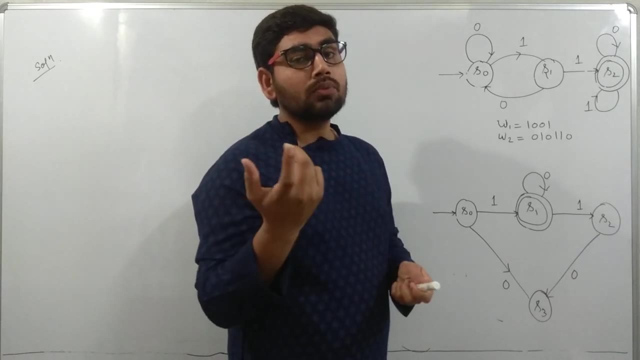 So we can say that S3 is a dead state. so in this type of language it gives zero input in the starting. No string can give such an input in which zero is coming. Such an input will be correct in which one is starting, Because it will go here after giving zero and we will reach the dead state. 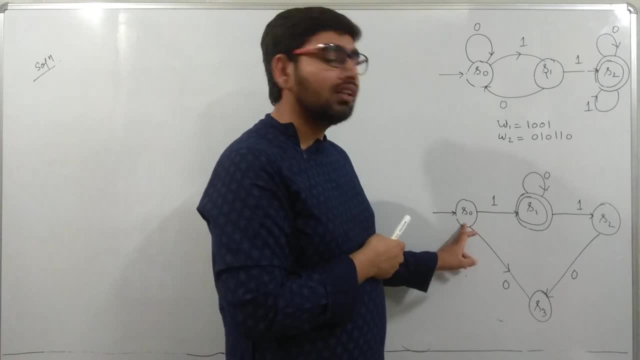 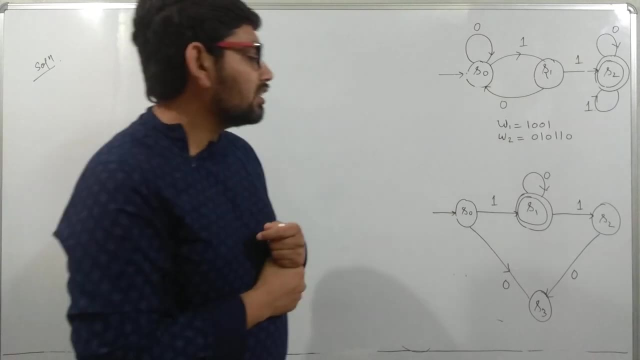 So we can't give zero in the starting. If we want to start S0,, then we will give one, So it will be accepted in this type of language. The first condition is starting from one. The second condition is that if we start from one, For example, we can't start from zero. 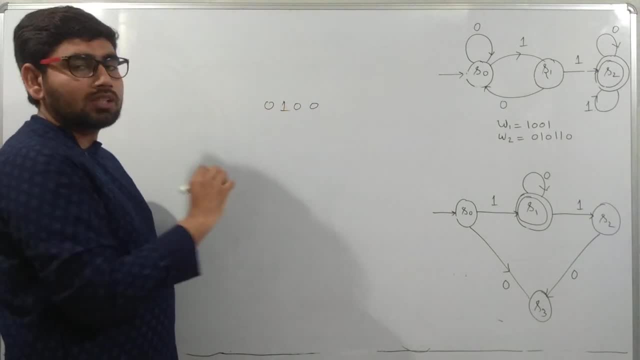 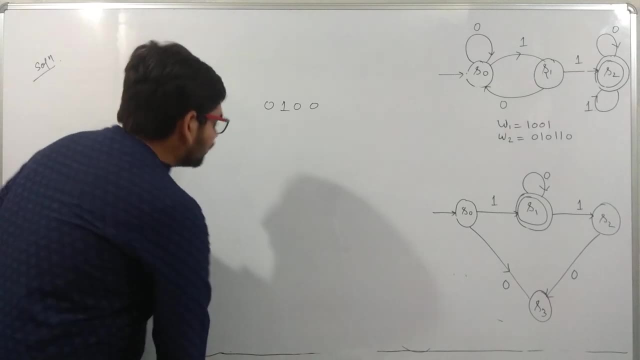 For example, if I want this string to be accepted in 0100, It will not be accepted because we have reached S3 from zero And S3 is a dead state, so we will not be able to move in it, So this type of string will not be accepted. 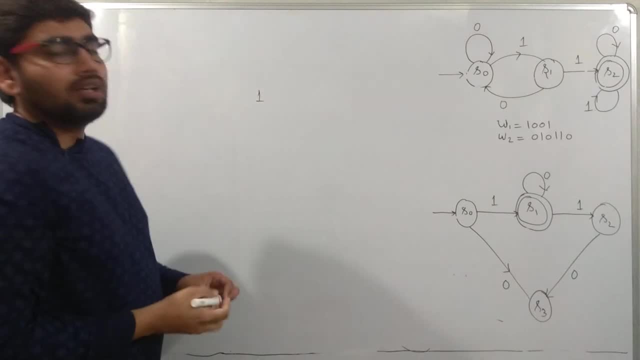 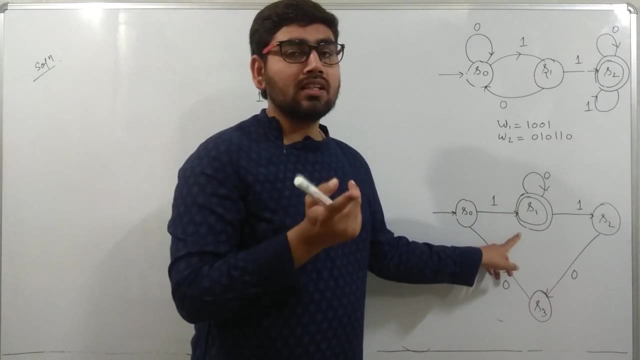 Which string will be accepted, in which one? We will start from one. We have stopped S0. When we will give one to S0, then we will observe that the accepting state is S1, And if we will give one to S1 again, then we will go to S2. 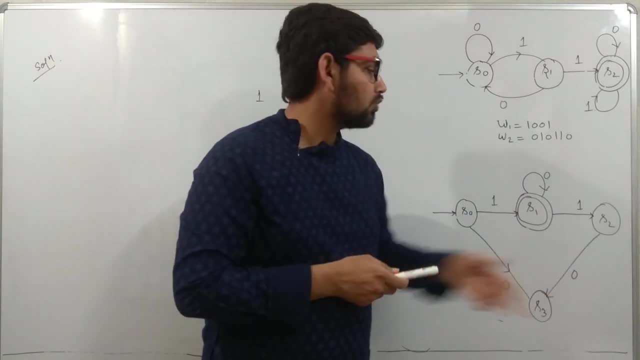 Now there is no way to go back from S2. If we will give S2 to zero, then we will go to S3. So S2 is also an unrecognized state. So we can go from S2 to S3, but we can't go back to S1. 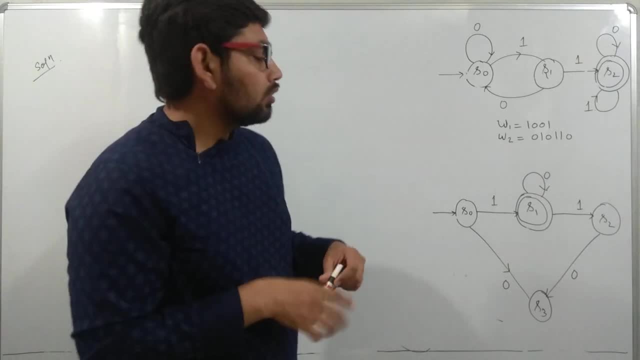 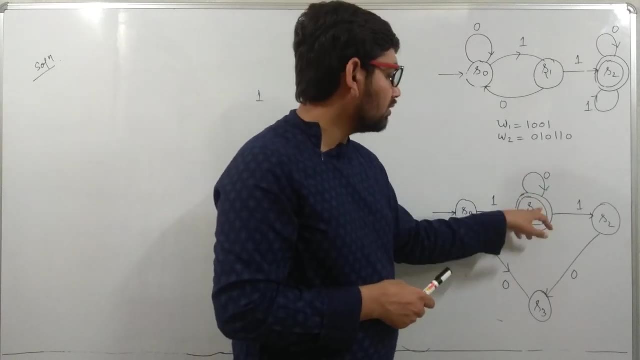 Means we can't accept our string. So our string will be accepted only when we have stopped it. Now we will give 0 to S1, So we will stay in S1. If we will give 1 to S1, then we will move to S1. 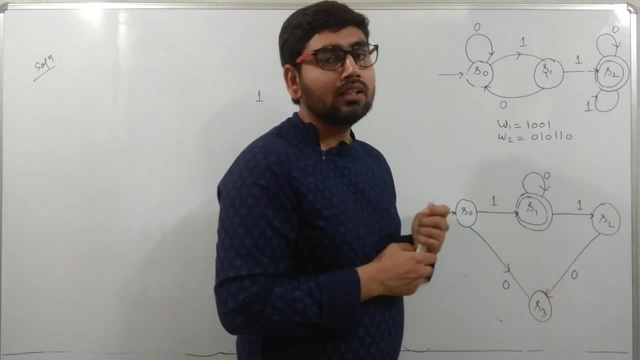 Then we will not be able to go back to S1. So, no matter how much we give 0 to S1, When we reach S1 state then we will get 0, But we should not get 1 again. If we get 1, then we will move forward. 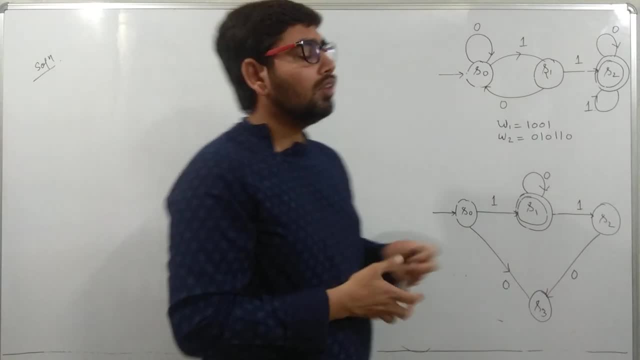 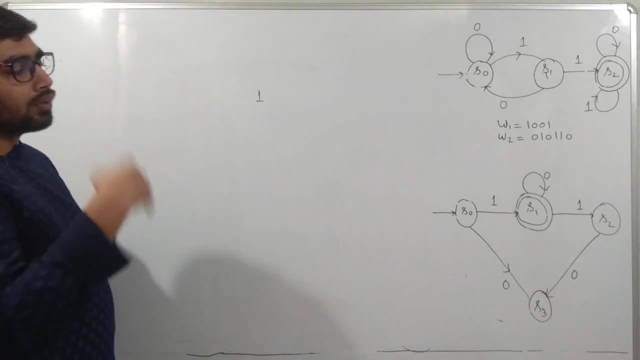 And we will not be able to reach this state again Because there is no arrow here. So we can conclude from here: We have to start from 1. If we will start from 0, then we have to reach the dead state. We have to start from 1. 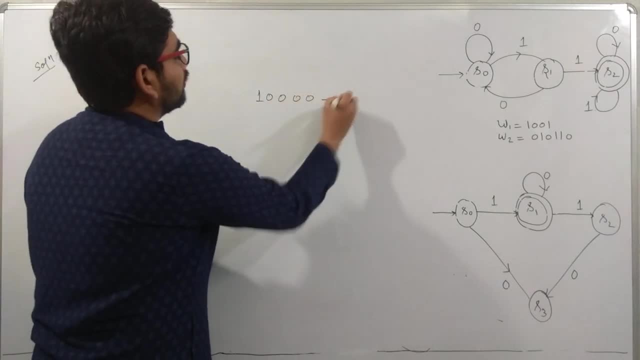 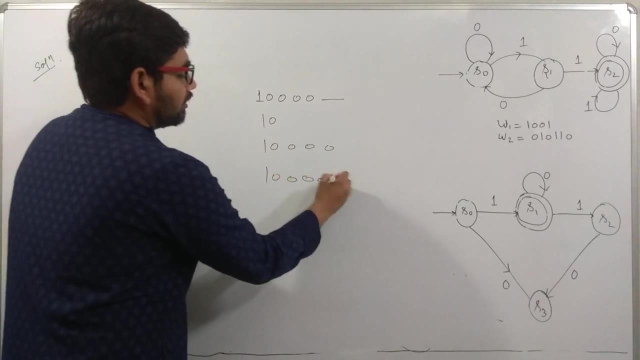 And if we will give anything further, then we can give 0. Any number of 0s can be here. This string will work. If we will give a single, then it will also work. This string will also be accepted. I will take this string and this will also be accepted. 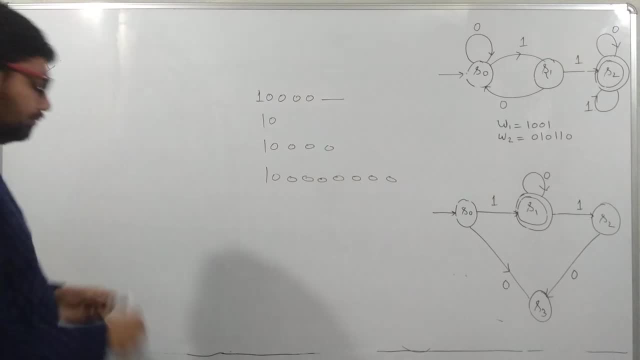 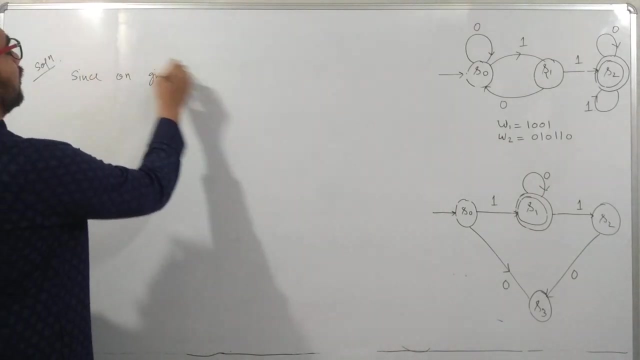 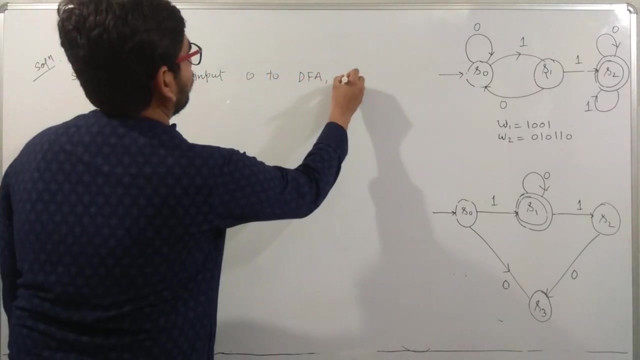 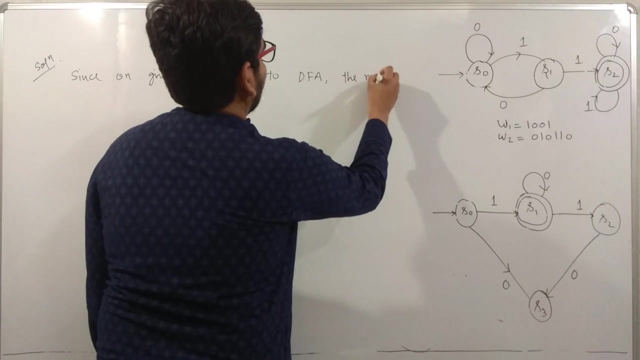 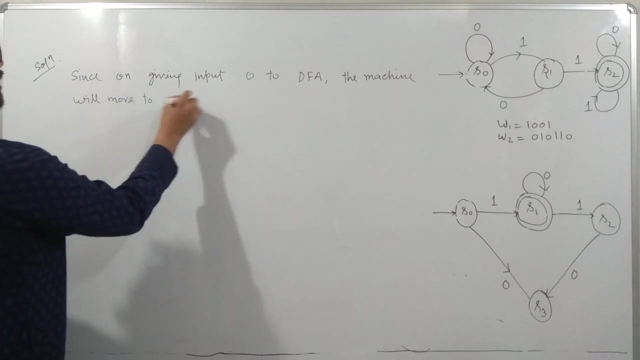 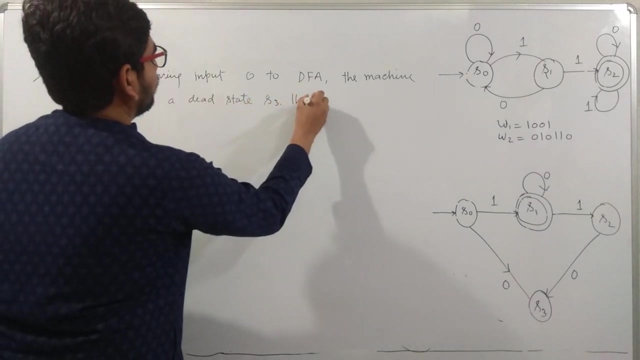 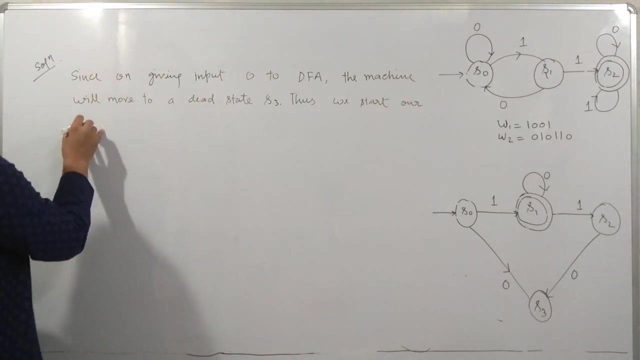 So all the strings will be accepted in this way. So we will define here, Since, On Giving Input 0 to DFA, The machine, The machine will move to The dead state. The machine will move to the dead state In S3. Thus We start Our input By 1.